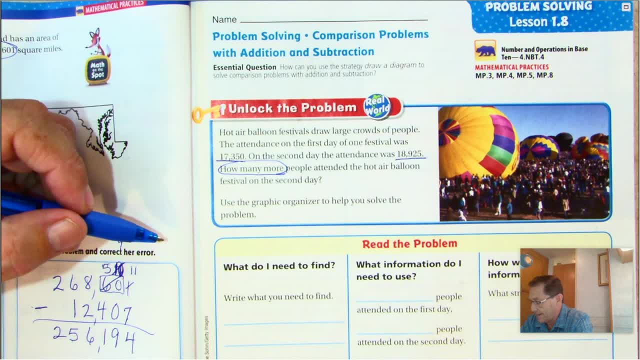 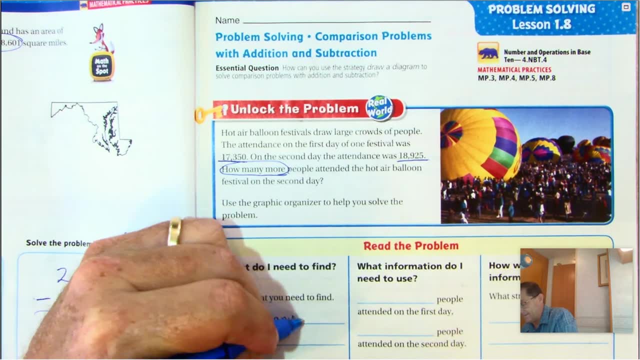 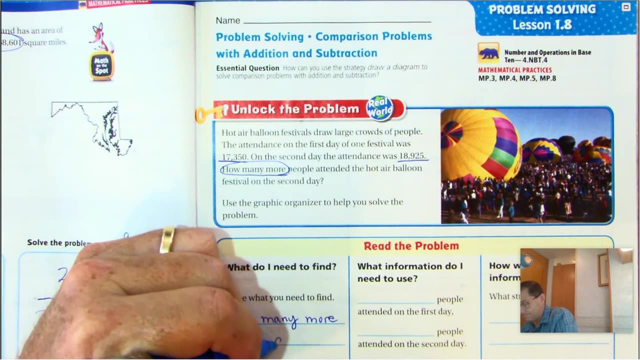 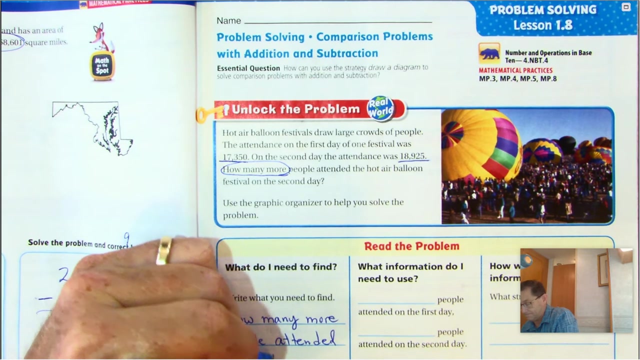 Use the graphic organizer to help you solve the problem. What do I need to find? How many more people? How many more people attended the second day? How many more people attended the second day? How many more people attended the second day? Then the first? 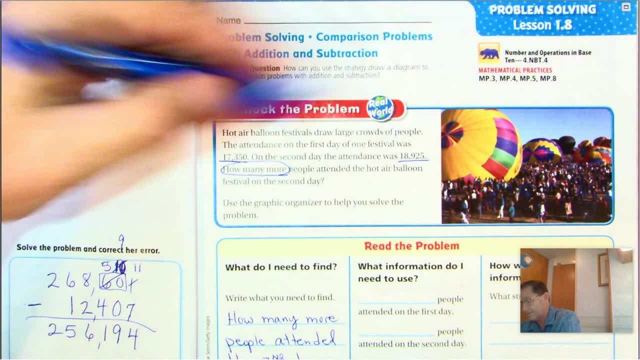 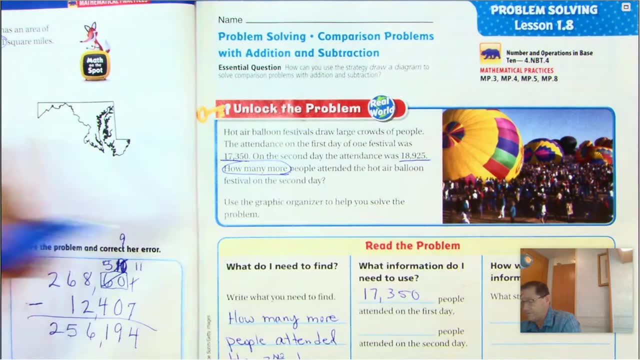 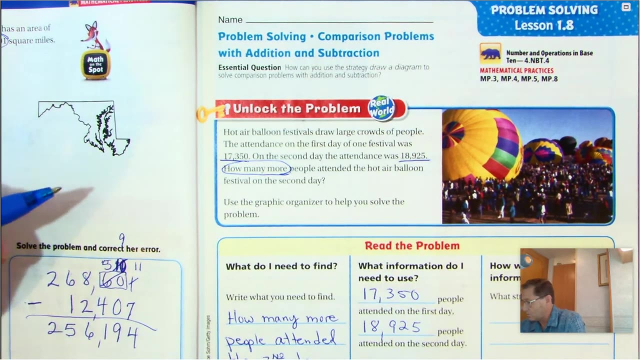 Okay, and what information do I need? So that's the information we circle: On the first day, 17,350 people attended and on the second day, 18,925 people attended. So how will I use the information? What strategy can you use? 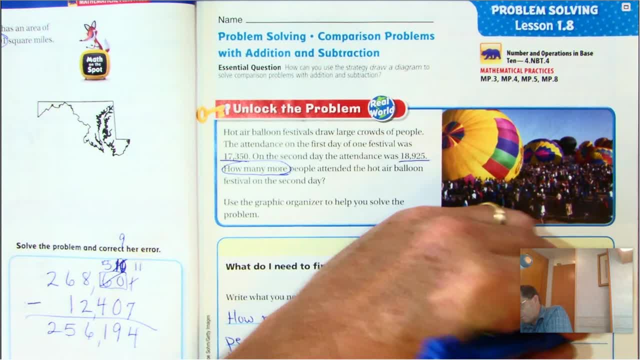 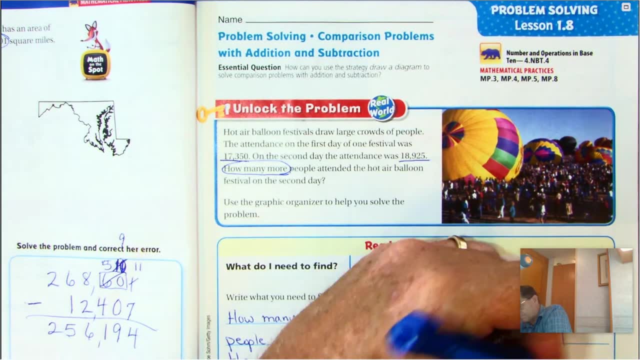 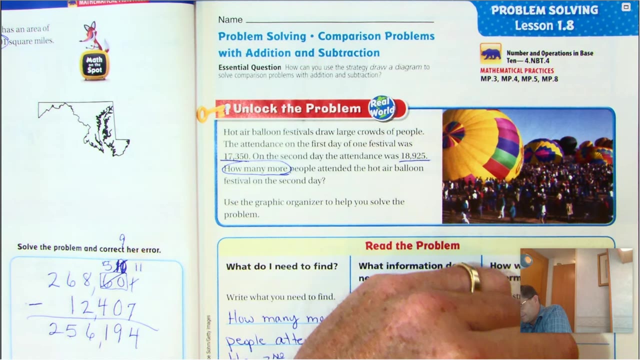 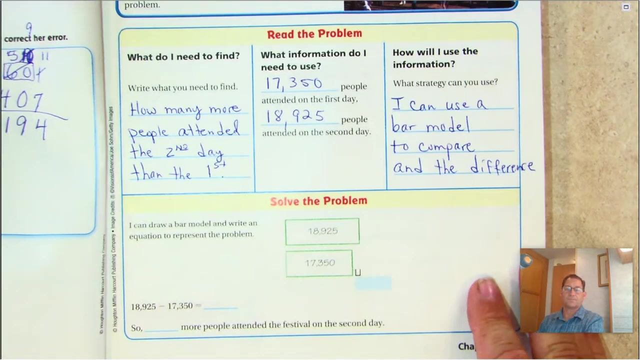 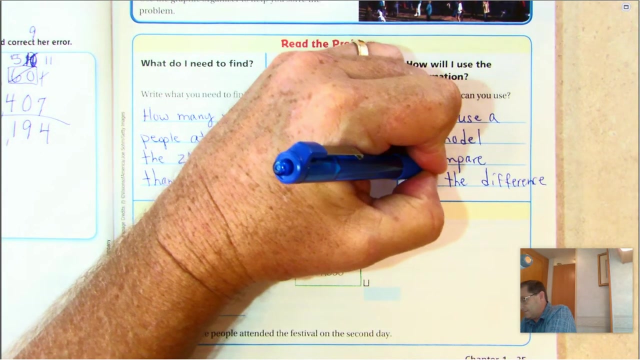 I can draw, I can use a bar model, I can use a bar model, I can use a bar model to compare and find the difference. So I can use a bar model to compare and find the difference And find the difference. Okay, so solve the problem. 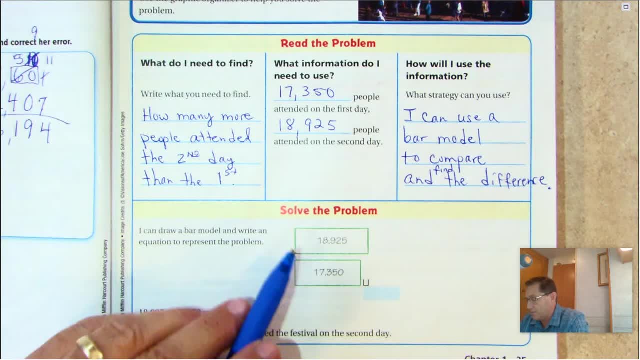 I can draw a bar model and write an equation to represent the problem. So we know that the second day there was 18,925.. We know that that is more than the first day. We know that that is more than the first day. 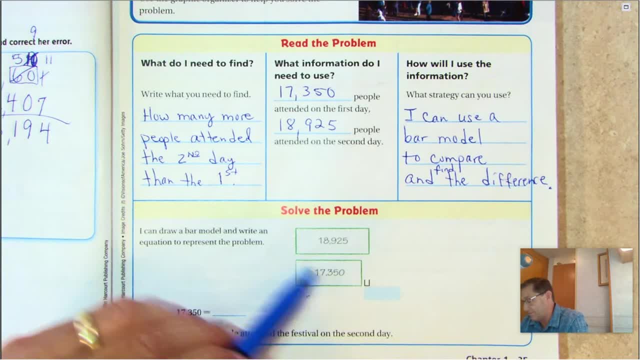 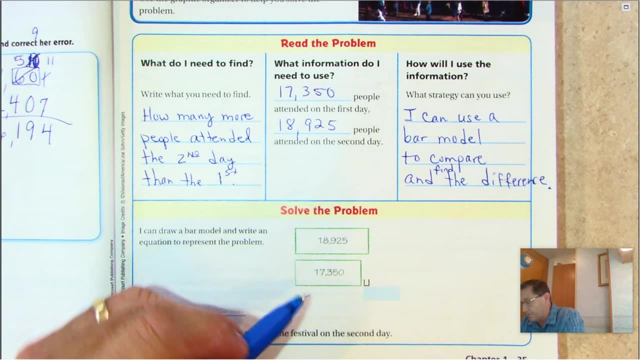 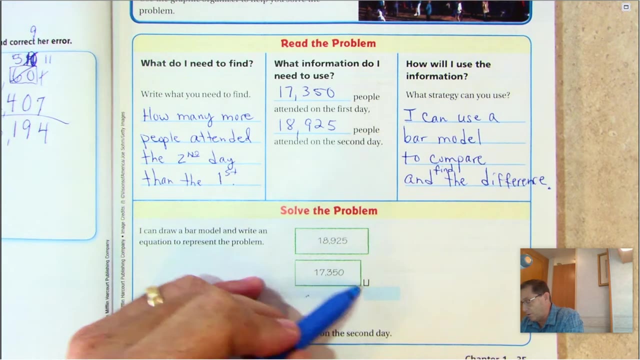 So if the second day, if the first day, was the same as the second day, it would be the same length as the first bump, But it's a little smaller, It has less people, And so we're showing this as a shorter bar in the first day. 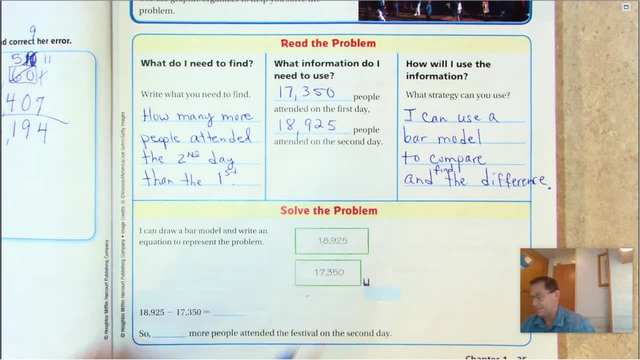 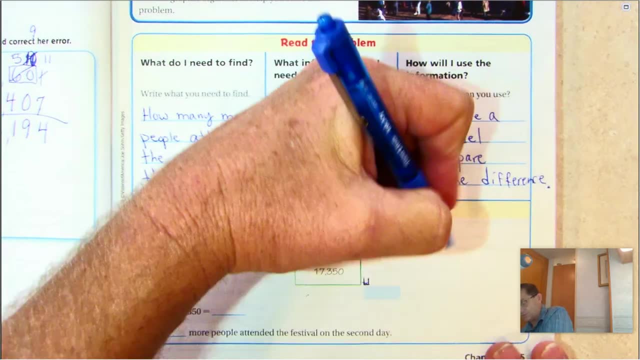 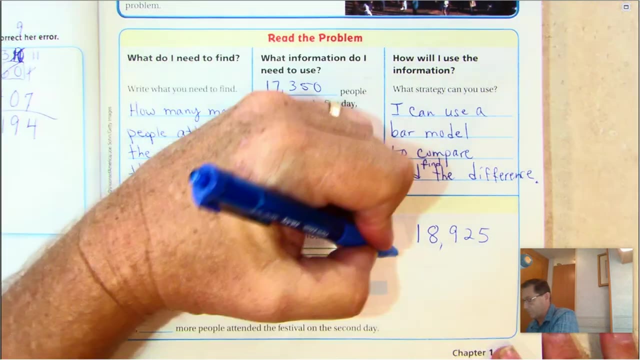 And so we're showing this as a shorter bar in the first day. And then this little space here represents how, And then this little space here represents how bigger the second day is. Okay, and so we're going to subtract to solve our problem. So we're going to take the second day, which was larger, and we will. 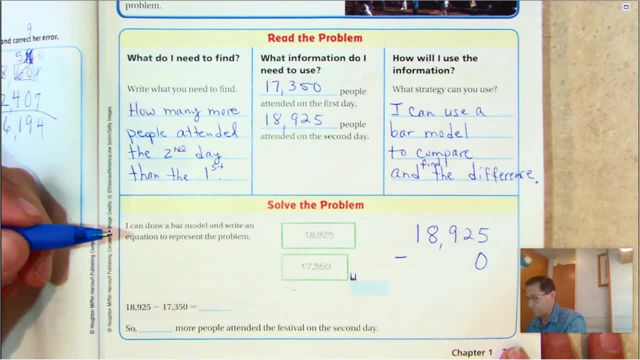 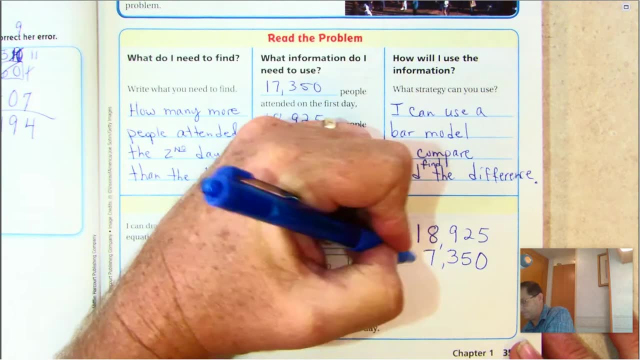 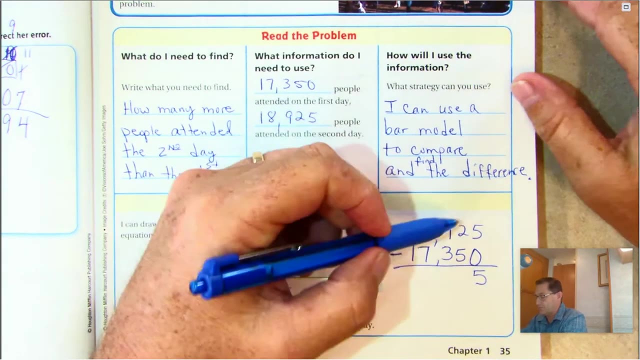 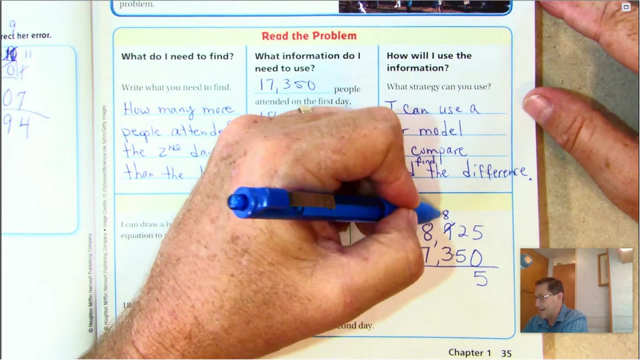 subtract. the first day We're going to line up our place value right to left, starting with the ones place. Okay, five ones, take away zero ones is five. Two tens, take away five tens. We can't do that, so we'll regroup and we'll trade the nine. 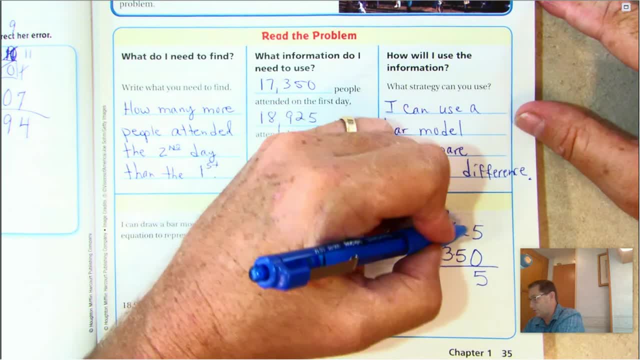 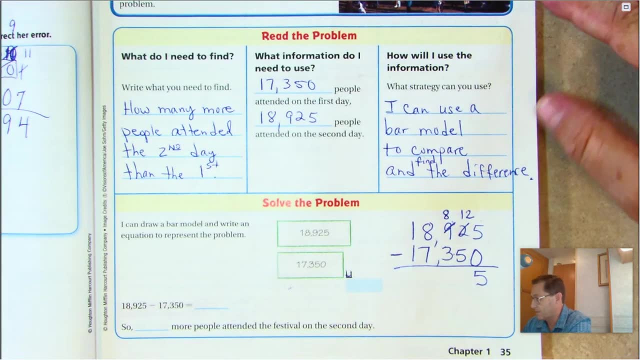 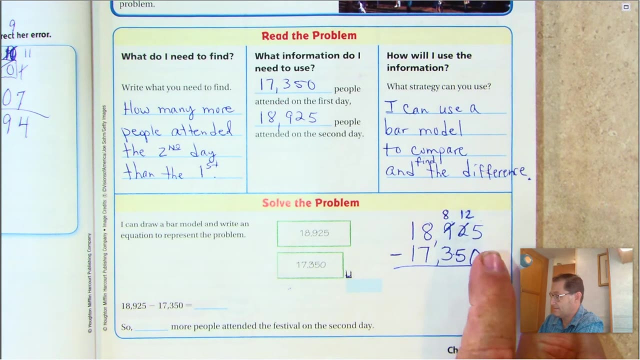 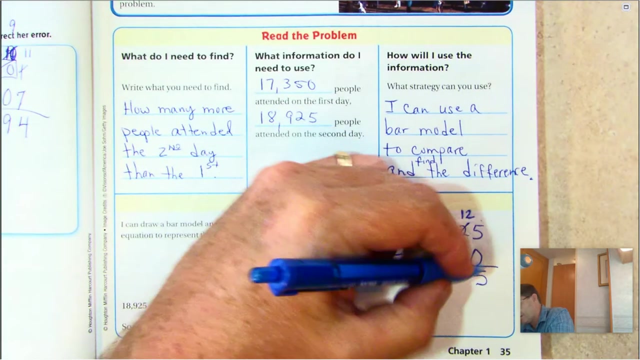 hundreds for 100, or eight hundreds and ten tens, And so we're trading the 92 tens for eight hundreds and twelve tens. Okay, twelve tens, take away five. tens is seven. Eight hundreds, take away. three. hundred is five hundred. Eight thousand, take away seven. 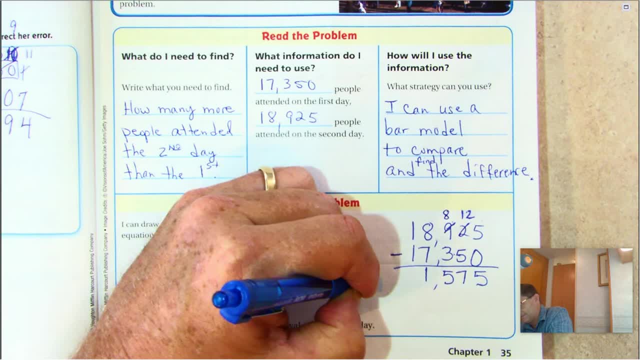 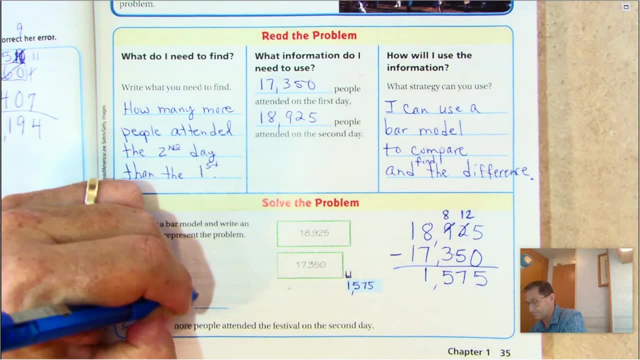 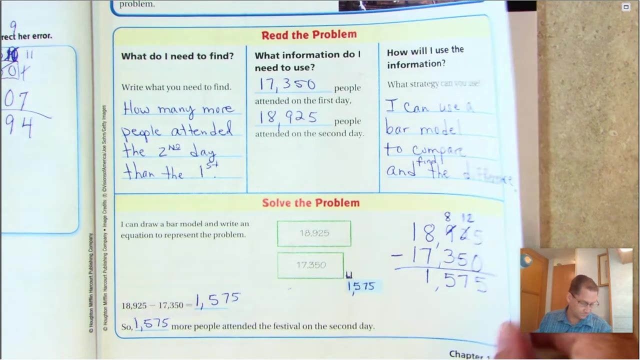 thousand is one thousand, So there's a little space. is one thousand five hundred seventy-five more people. Okay, we're going toDDO. so the higher 10s, the higher tens take far the more is, the longer it takes to run. uh, hour out and the baseline is rather short And this: 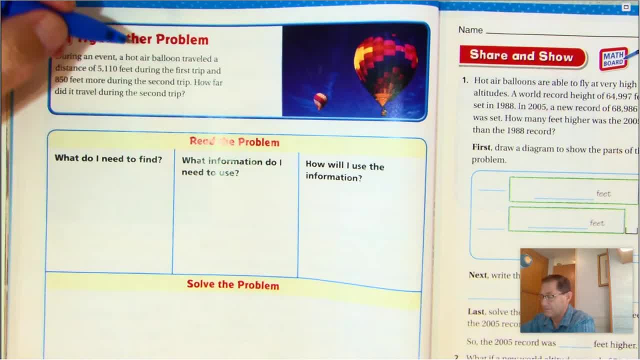 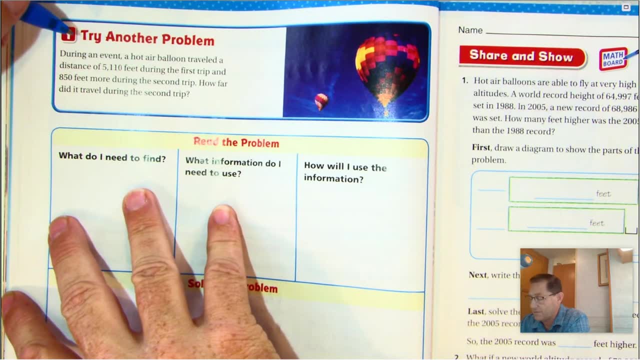 goes everywhere, So we're going to take on the probability thatariat times вамьão's massa is auctioned. Okay, turn to page 36,. During an event, a high-air balloon traveled a distance of 5,110 feet during 107,れ. 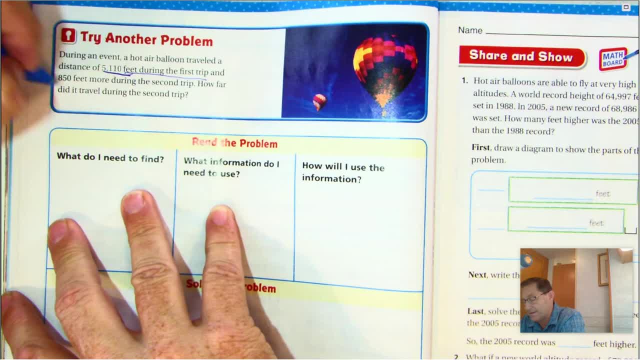 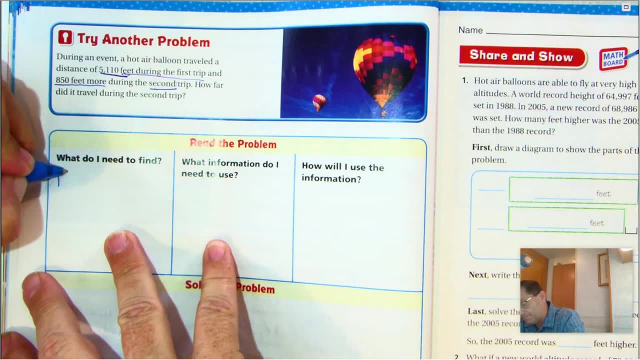 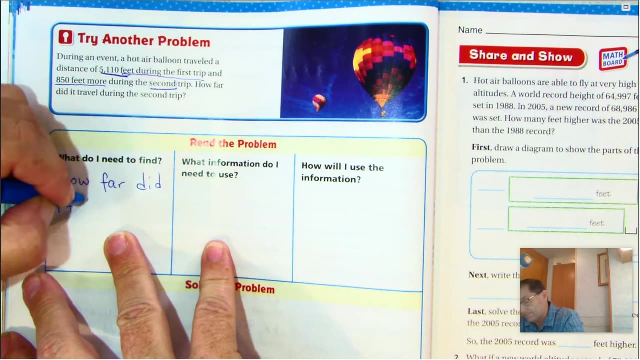 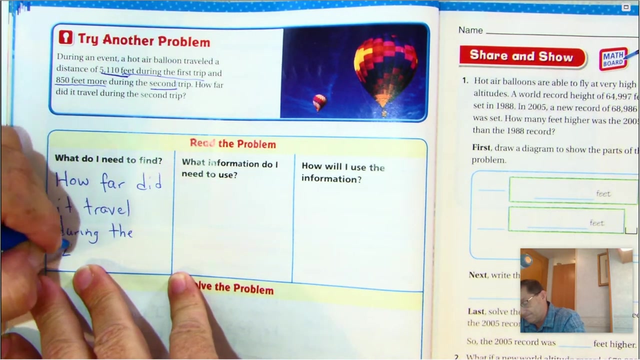 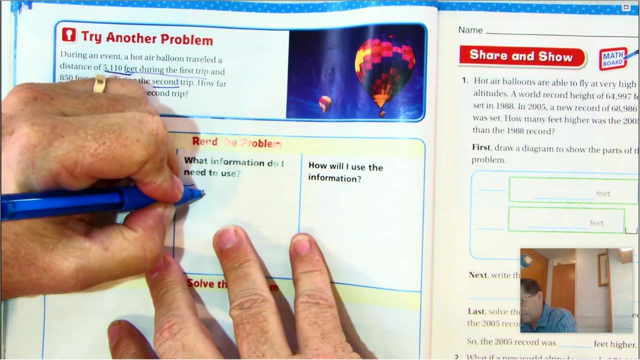 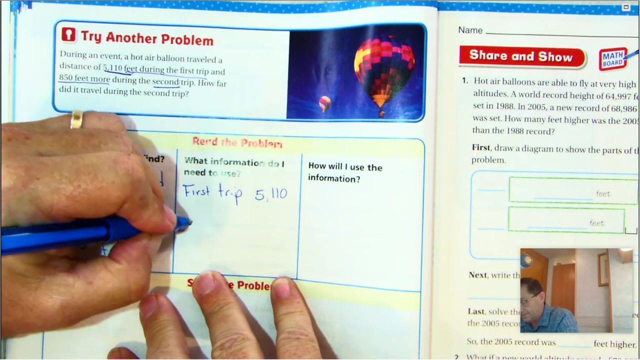 5,000 during the first trip, 850 more on the second trip. So what do we need to find? We need to find: how far did it travel during the second trip? What information do you need to know? First trip: 5,110 feet. Second trip: 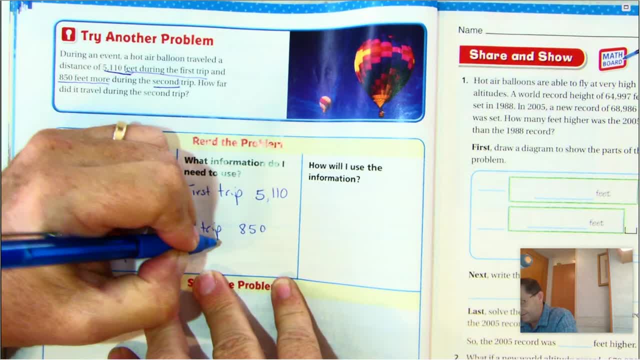 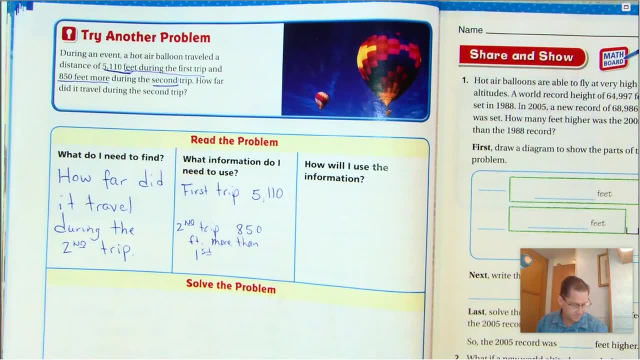 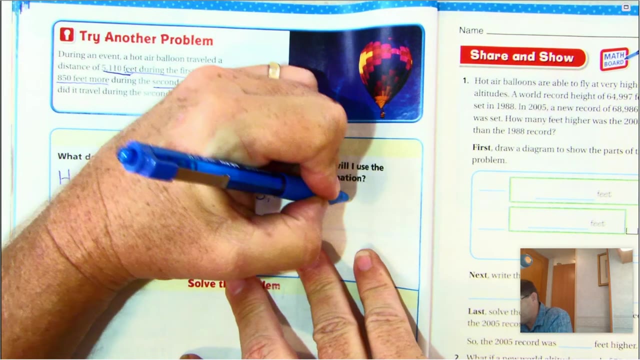 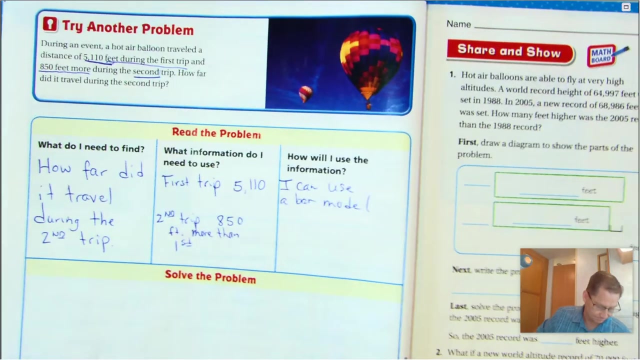 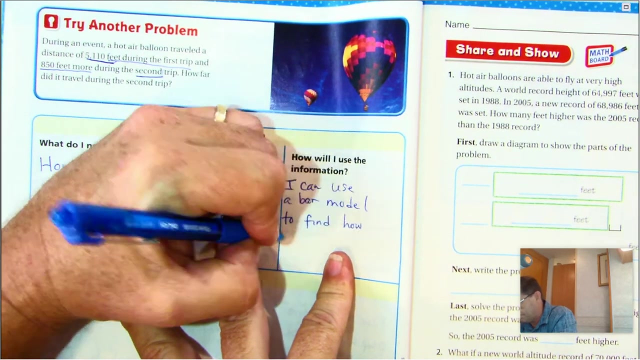 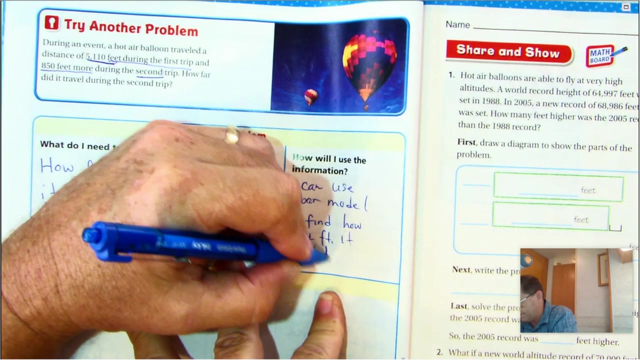 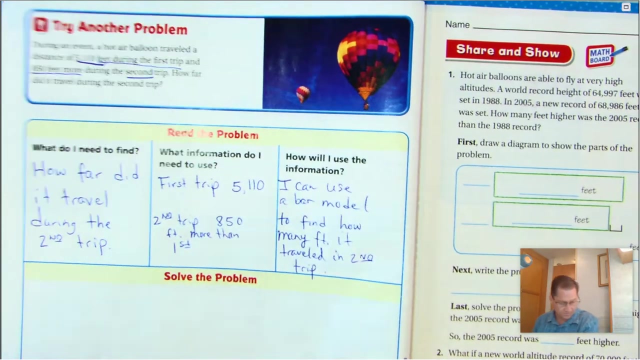 850 feet more than first. So what can we use? You can draw a diagram or use a bar model. How many feet did it travel in the second trip? Okay, so now we're going to solve the problem. So what do we need to know? We need to know how far did it travel during the second trip. 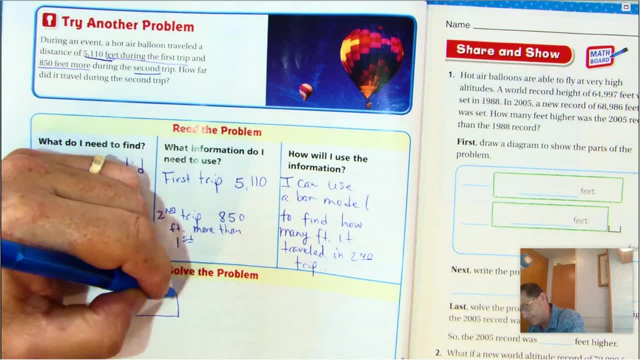 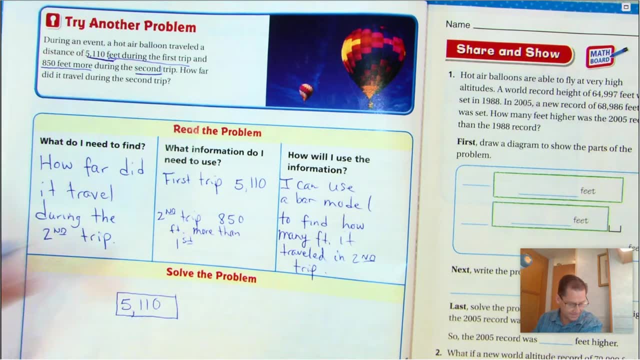 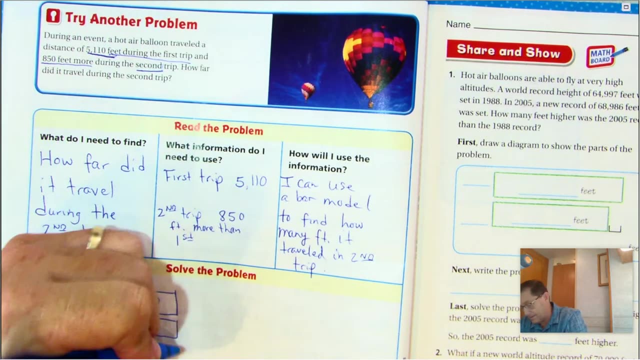 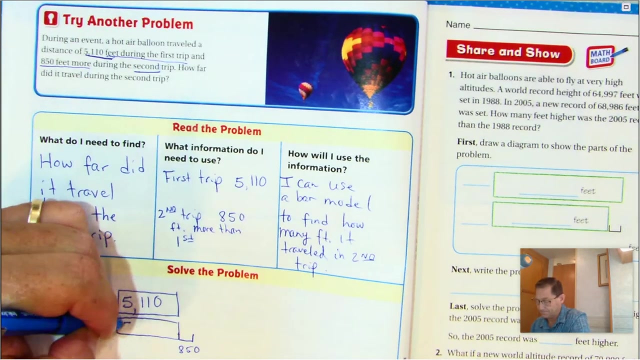 What information do you need to know? We need to know how far did it travel during the second trip. We know that the first trip was 5,110 feet And the second trip was that same 510 plus 850.. So what do we need to know? We need to know how far did it travel during the second trip. 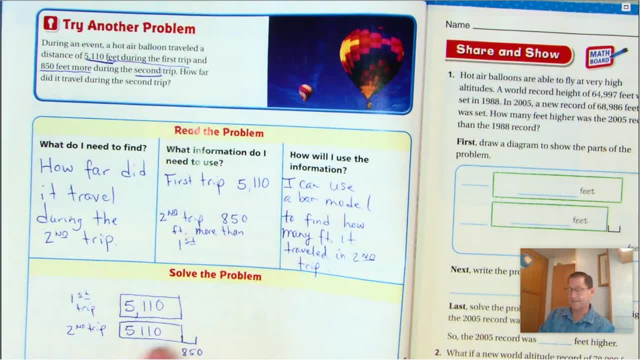 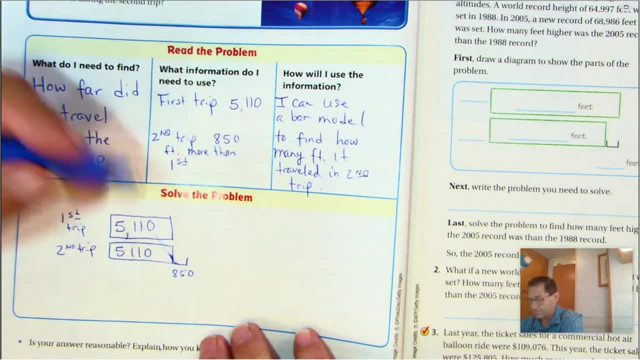 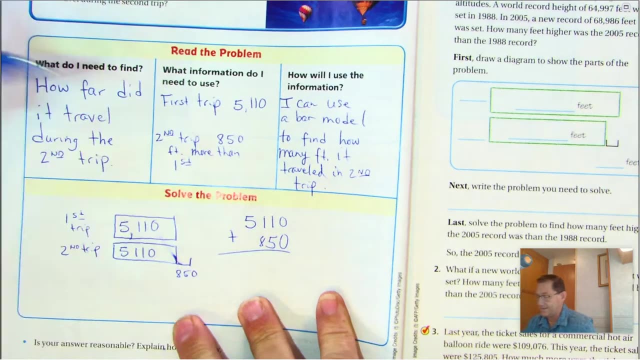 We need to know how far did it travel during the second trip. So we know that second trip has to be slightly bigger than the first trip because it was 850 more feet. So this we're just going to add the additional 850.. 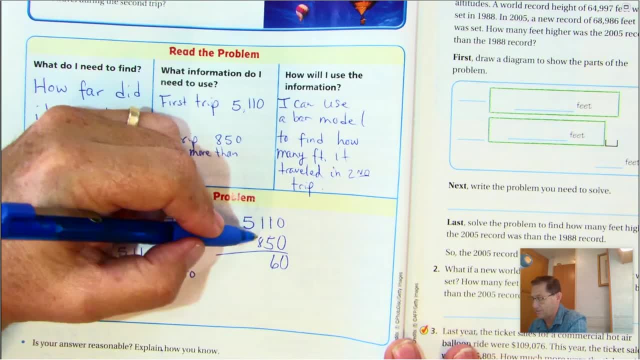 Zero ones plus zero ones is zero. 5-tens plus one ten is six tens. 800 plus 100 is 900, and 5,000 plus nothing is 5,960.. Here we go: 800 plus 100 is 800.. 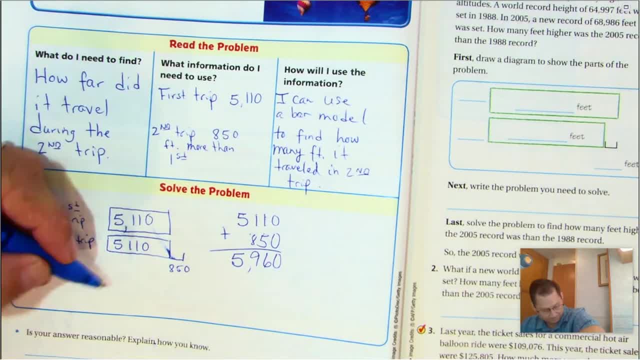 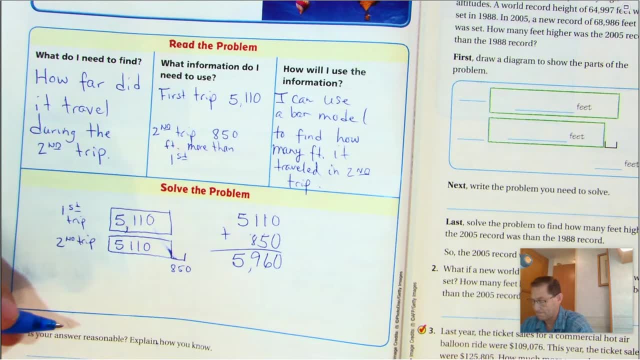 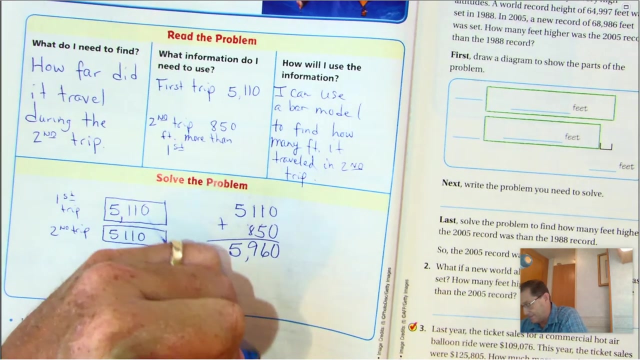 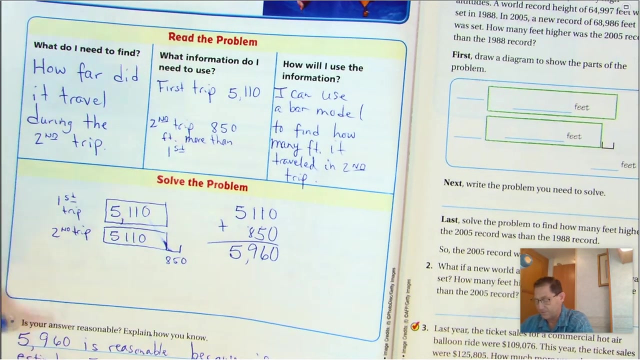 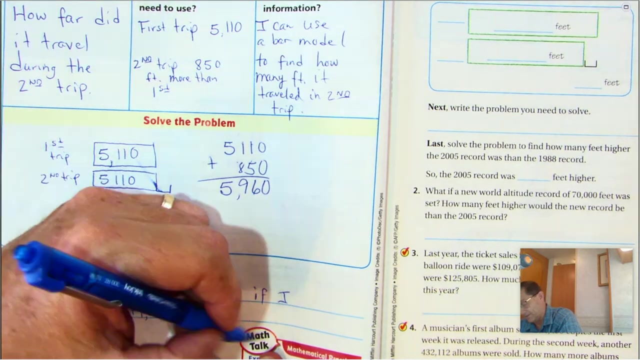 We have to start with 850, then add 9,000.. 5,960 is reasonable because if I estimate 5,000 for the first trip plus about a thousand for the second trip, it would be about 6,000 feet. and so five five thousand nine hundred sixty is close to six thousand. 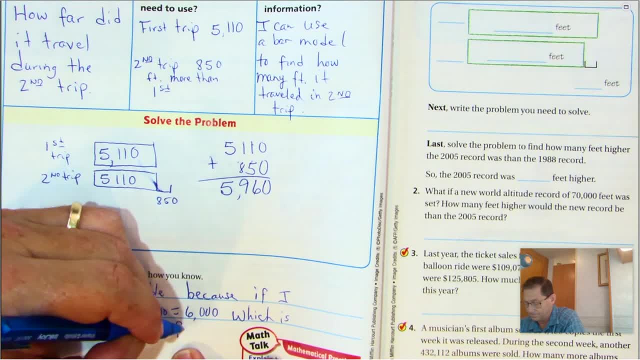 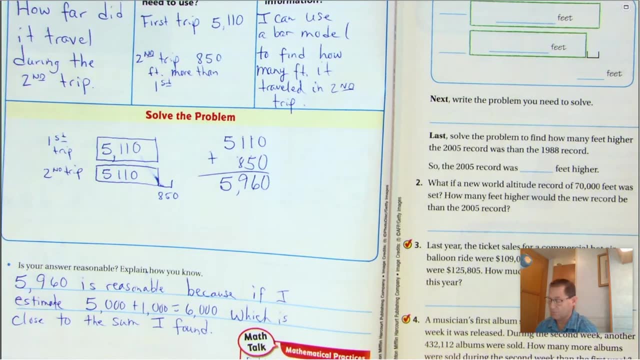 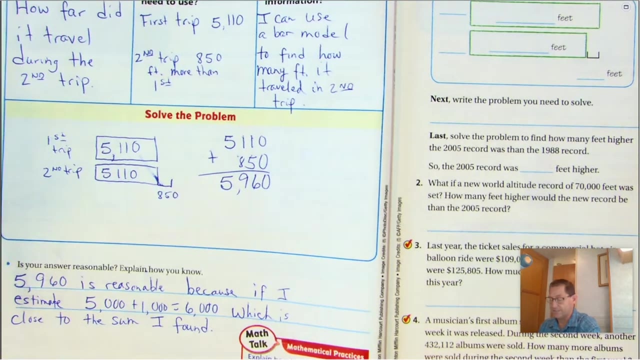 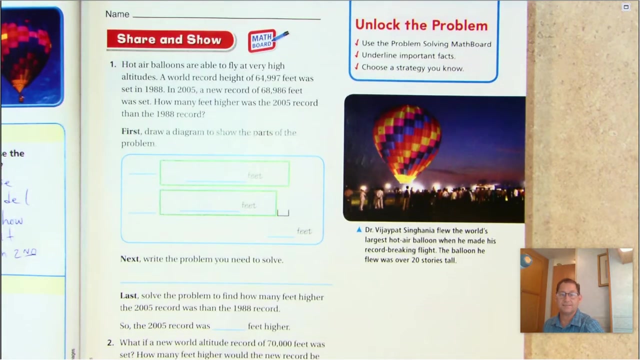 five thousand nine hundred sixty is reasonable because if I estimate 5,000 plus 1,000, first trip plus second trip, I get to 6,000, and 6,000 is close to the sum I found of 5,000. okay, so now Sharon's Joe, let's practice these. so one. hot air balloons are able to fly a very high altitude of world record height of 64,000 997 feet. was that in 1988? in 2005, a new record of 68,000 986 feet was set. how many feet higher was the 2005 record? 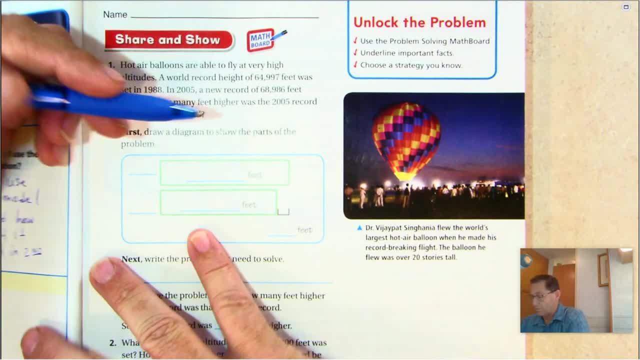 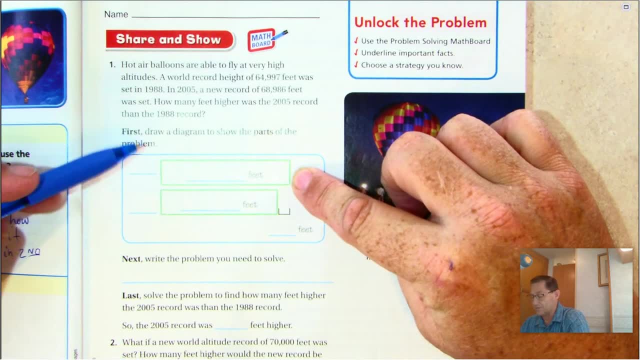 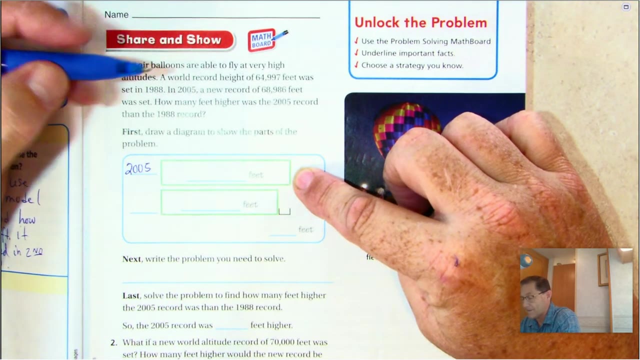 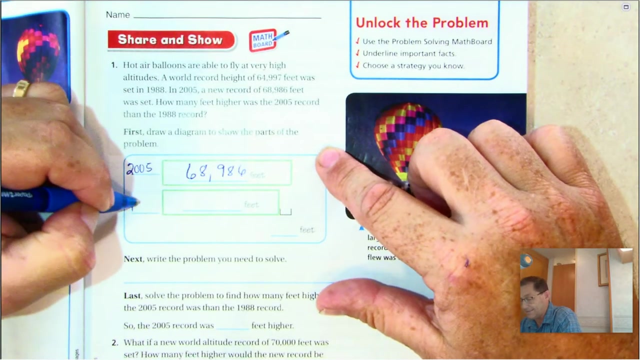 than the 1988 record. so I look at my drawings here and the longer box would be the 2005. So in 2005, it was 68,986 feet, which was bigger than the record of 1988, which was 64,997.. 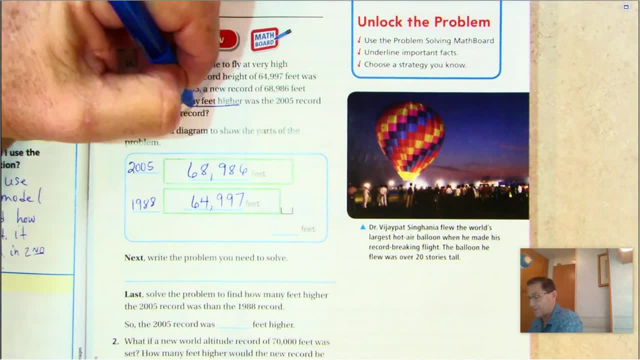 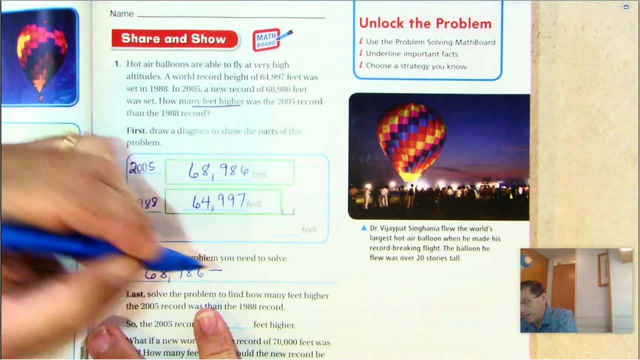 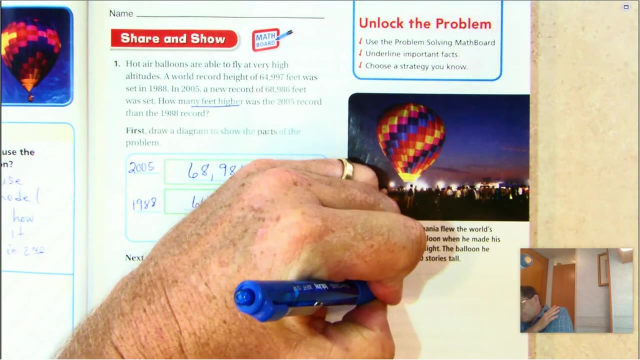 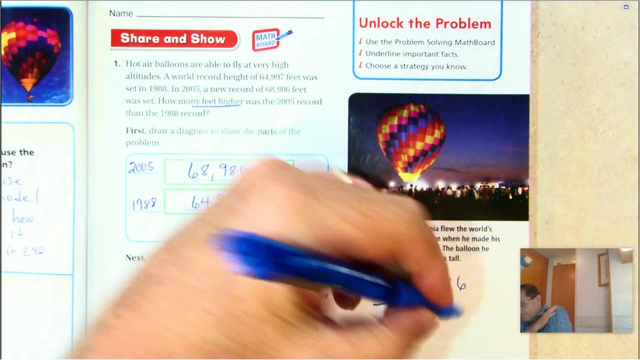 So we need to find how many feet higher We need to solve 68,986,, take away 64,997.. Start with the greater number and subtract the smaller value. Okay, I'll make sure that I've lined up each of the place values, and they do. 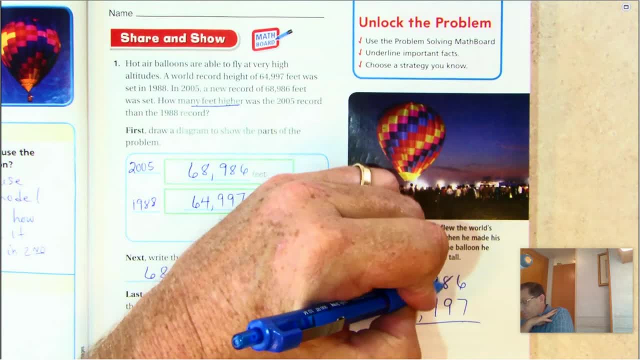 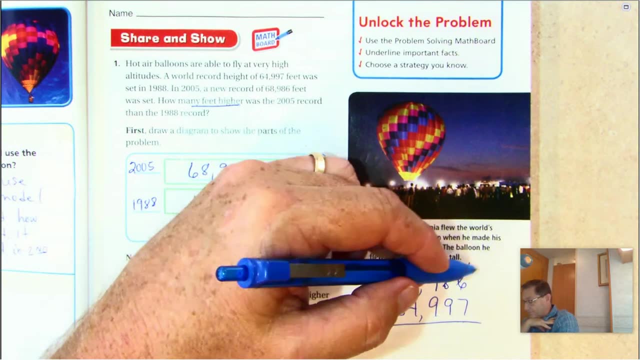 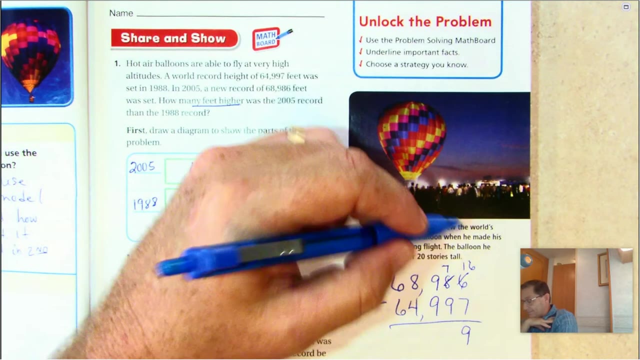 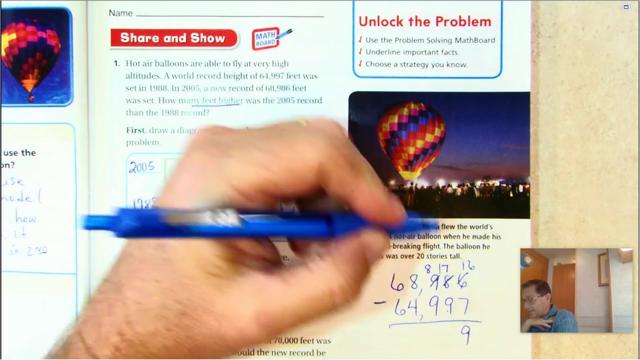 I can't take seven ones from six ones, So I'll regroup the eight tens as seven tens and one ten Ten ones. Eight tens as seven tens and ten ones. 16 take away seven is nine. Seven tens. take away nine tens. I can't do so. I'll rename the nine hundreds as eight hundred and tens. 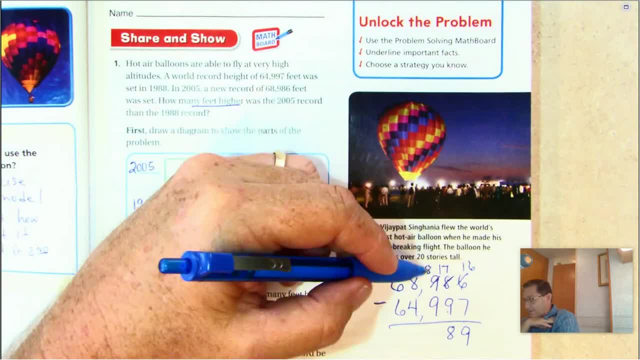 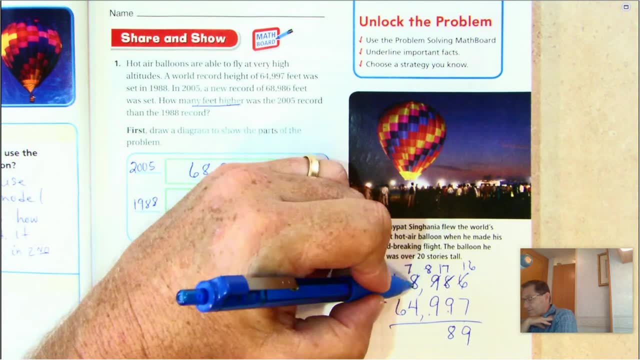 17 take away nine. tens is eight tens. 800 take away 900.. I have to rename from there 8,000, 8,000 can be renamed to 7,000 and 10 hundreds. 18 take away 900 is 900.. 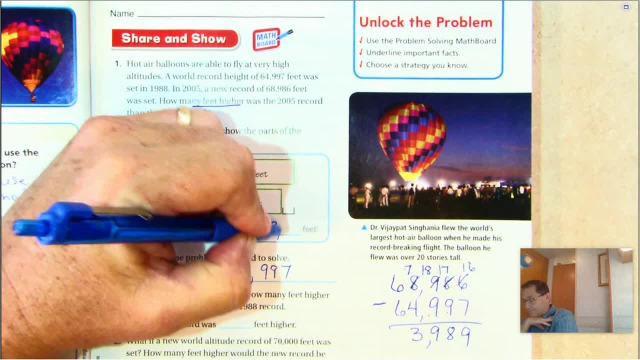 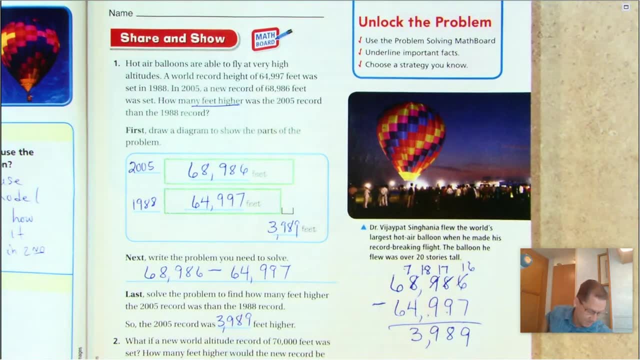 7,000. take away four is three, So it was 3,989 feet higher. But what if a new world record was set of 70,000 feet? How many feet higher would the new record be than the ten? How many feet higher would the new record be than the two thousand and five? 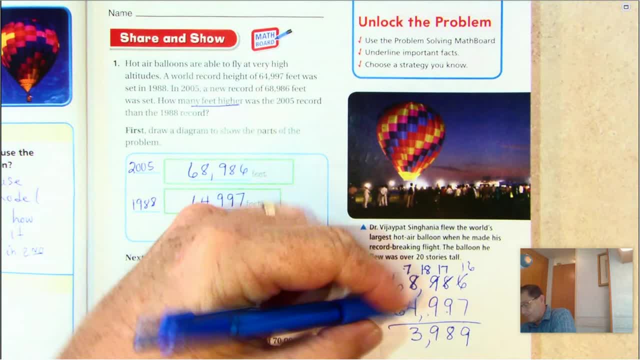 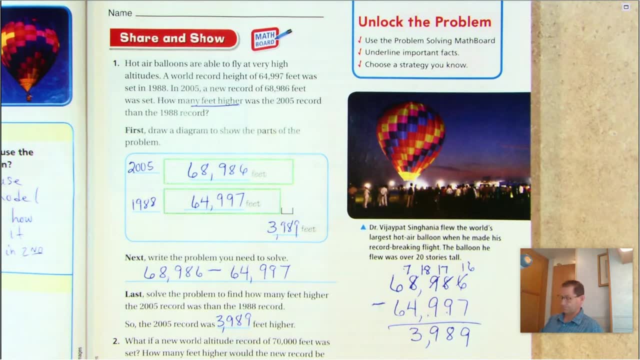 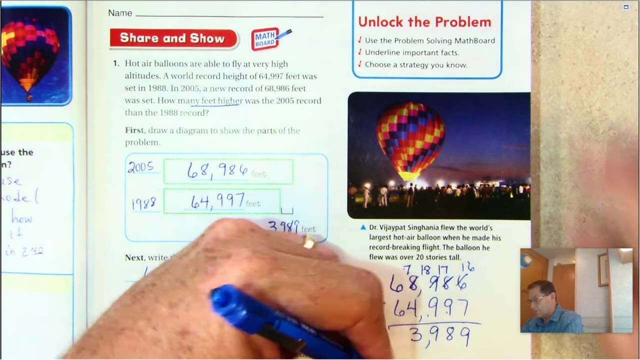 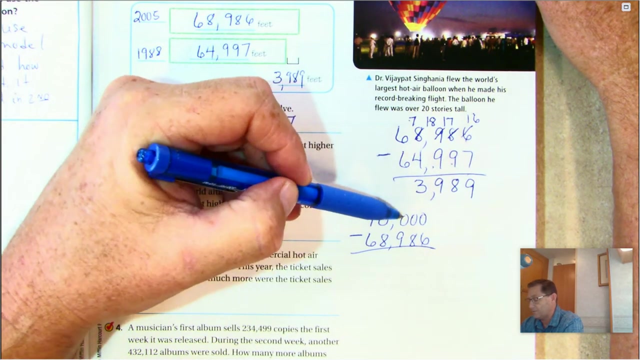 So this time we have 70,000, take away 68,986.. So I can't take six ones from nine. There's no tens to regroup, There's no hundreds, There's no thousands. So I'm going to start with regrouping. 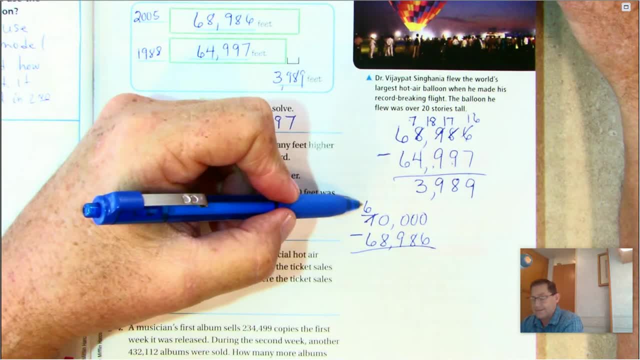 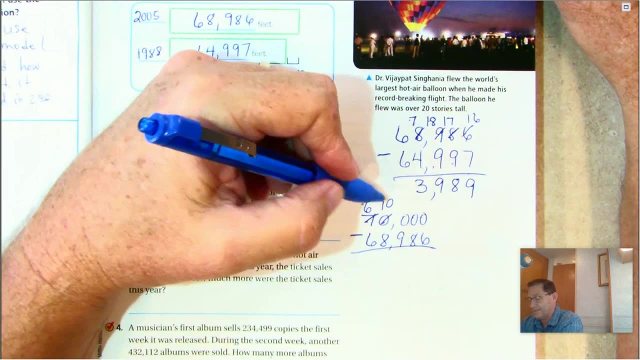 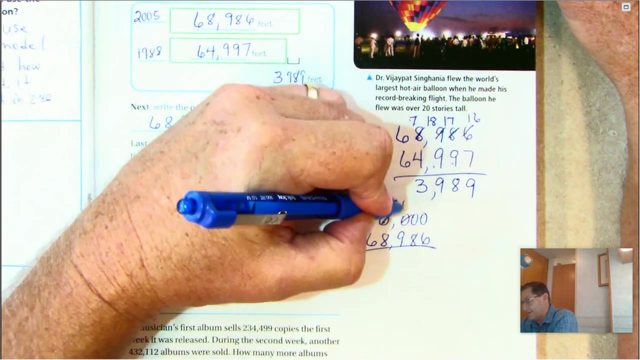 Regrouping from the ten thousands. I'm going to rename the ten thousands as 6,000.. Six, ten thousands and ten thousand ones. I can rename the ten thousand ones as nine thousands and ten hundreds. I can rename the ten hundreds as nine hundreds and ten tens. 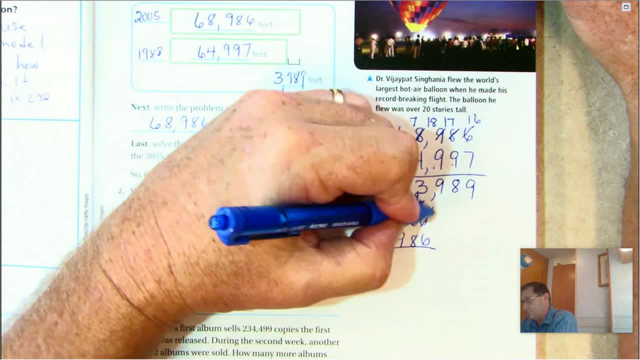 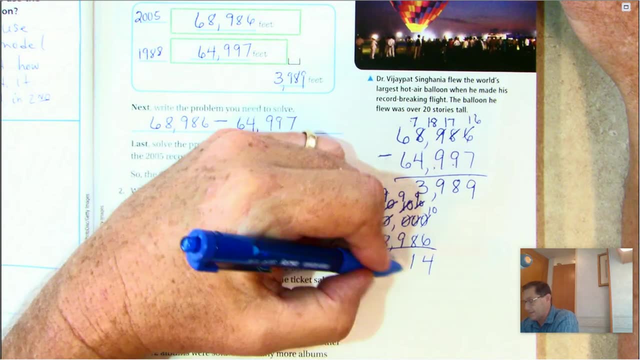 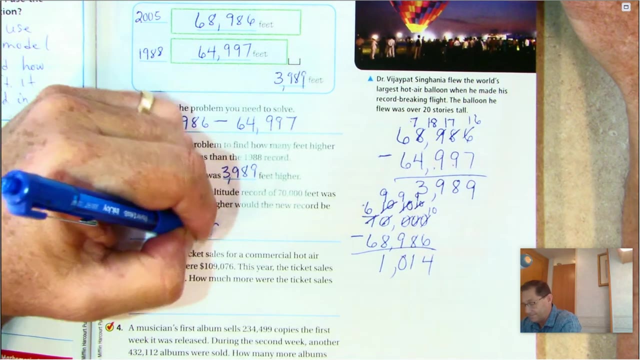 I can rename the ten, tens as nine, tens and ten ones. So ten take away six is four. Nine. take away eight. tens is one. Nine hundred take away nine, hundred is zero. Nine thousand take away eight thousand is one thousand. So it would be a thousand fourteen feet higher. 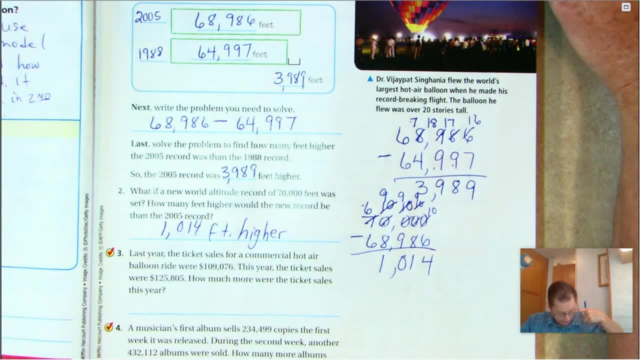 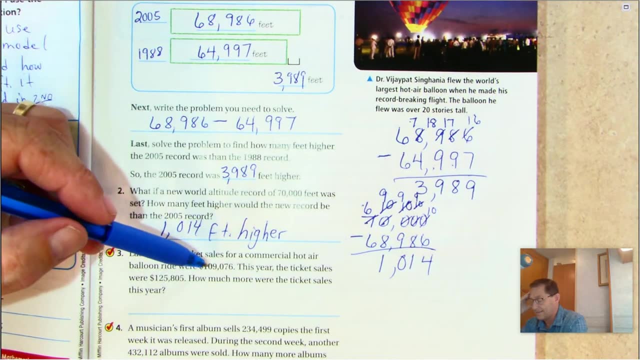 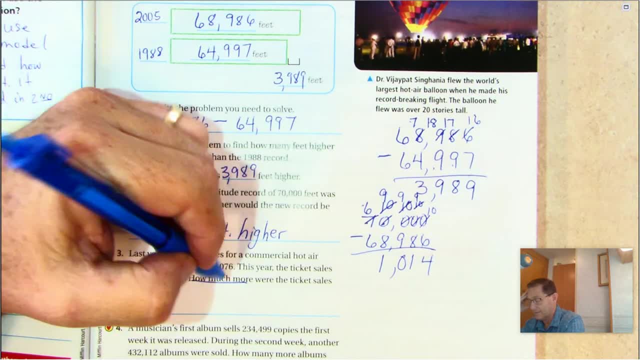 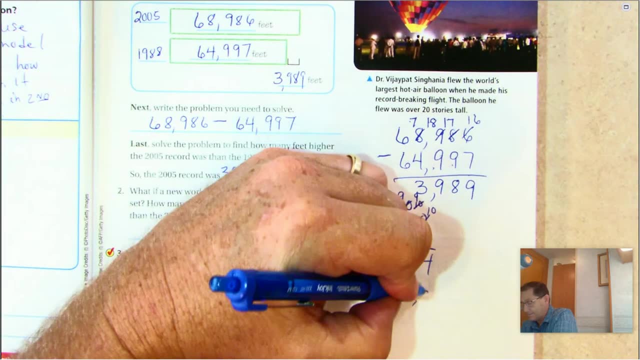 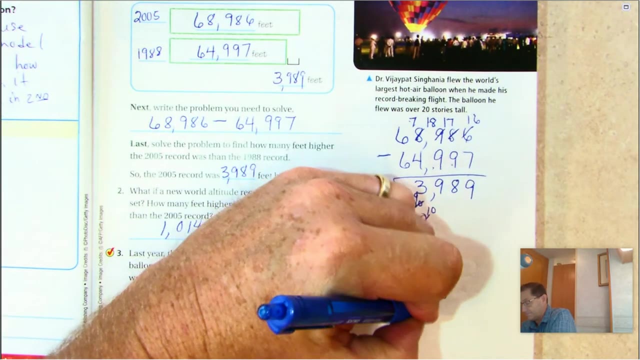 This year the ticket sales were $125,850.. How much more were the ticket sales this year than last year? We have $125,805.. I'm going to subtract the amount of the previous year to find out how much more money was made. 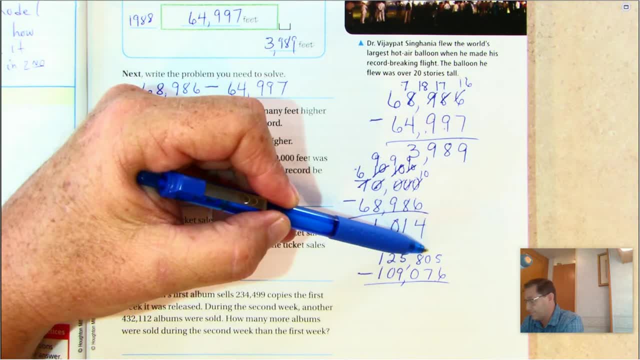 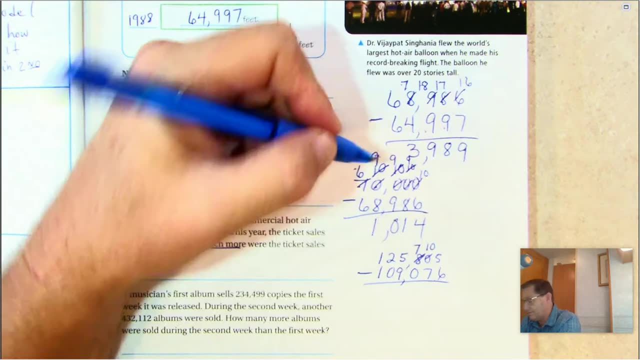 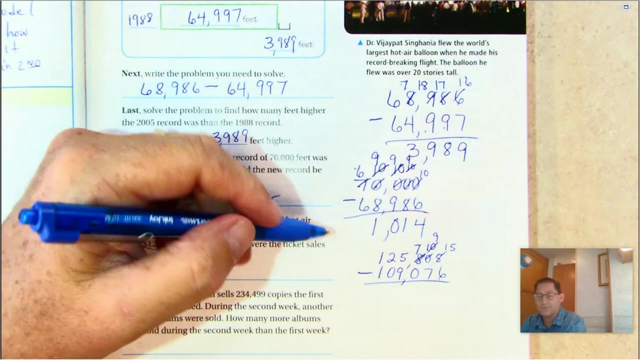 I cannot take six from five. There are no tens to regroup. Eight hundreds as seven hundred and ten tens. Now I can rename the ten tens as nine tens and ten ones. Fifteen take away. six is nine. Nine tens take away seven. tens is two. 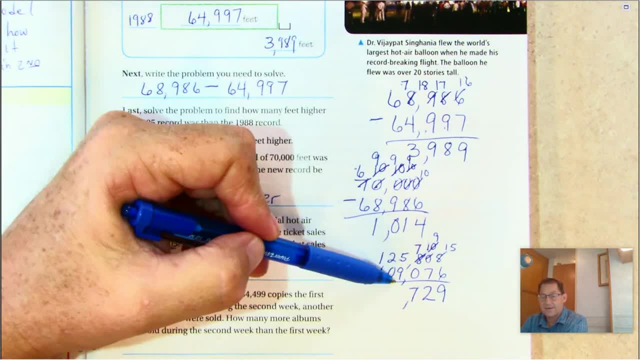 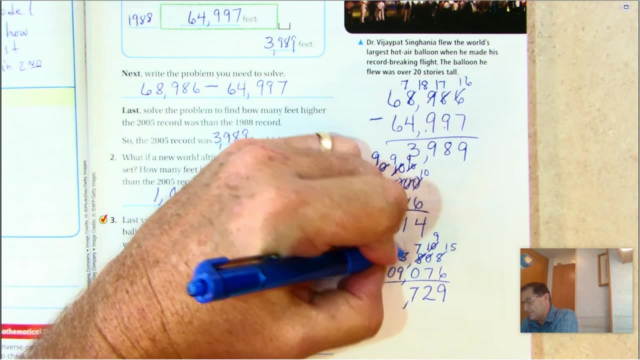 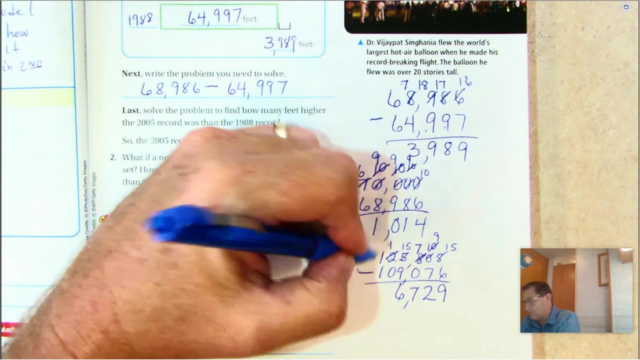 Seven hundred, take away no hundreds is seven. Five thousand. take away nine thousand. I can't do, But I can rename the two, ten thousands as one ten thousand, Ten, ten thousand and ten one thousand Fifteen. take away. nine is six. One ten thousand, take away. nine is one. 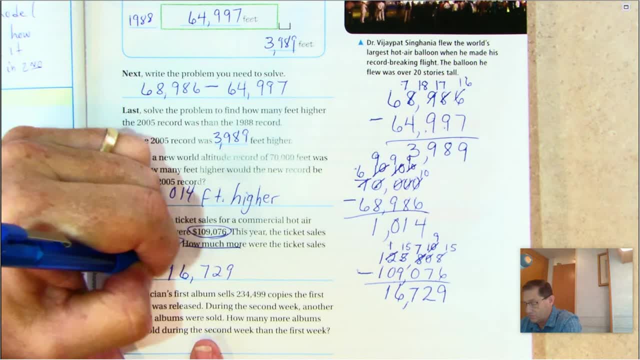 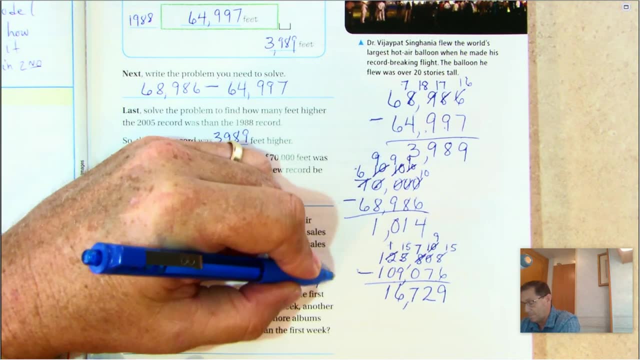 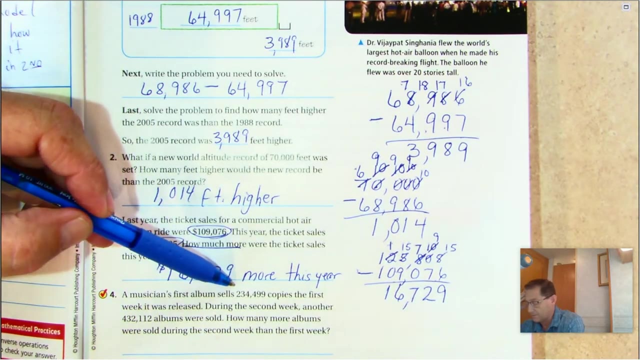 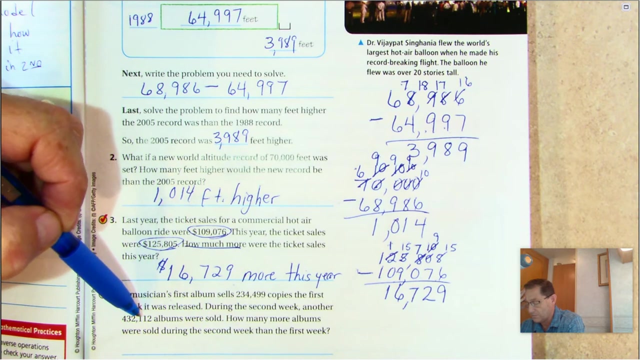 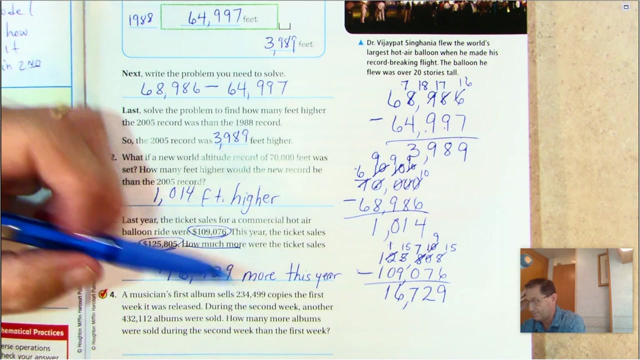 So it's $16,729 more this year. A musician's first album sells 234,499 copies the first week it was released. During the second week, another 432,112 albums were sold. How many more albums were sold during the second week than the first? 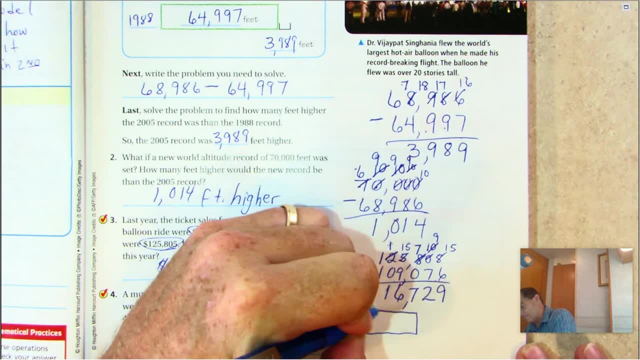 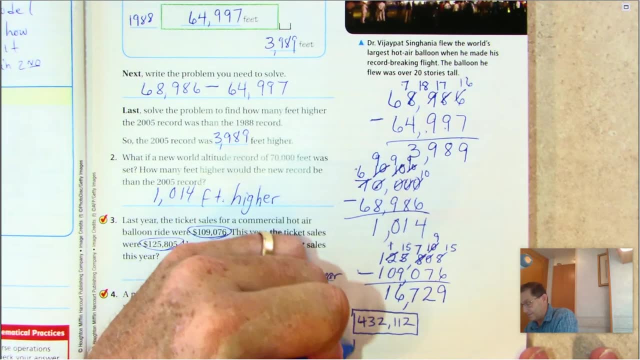 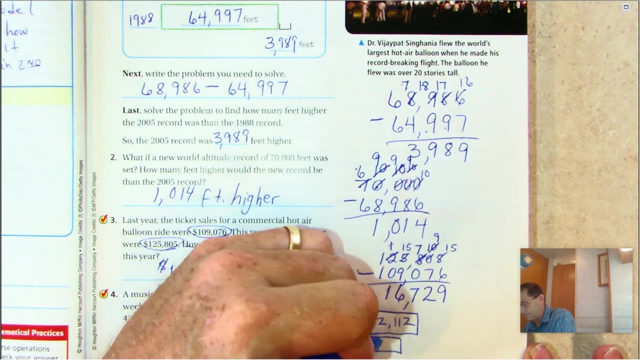 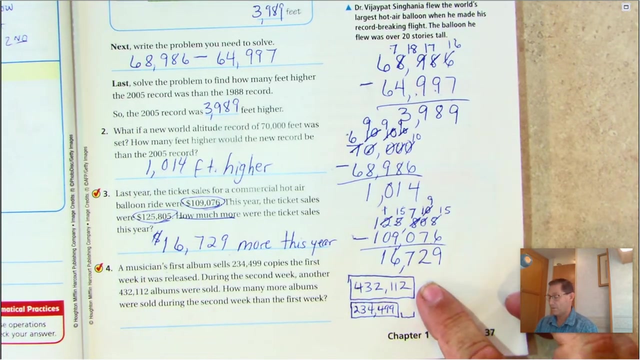 So this is my second week And the first week is not going to be as long because there was not as many records sold or albums sold, But we need to find out how much more or how much is missing from the first week. that would have made them equal. 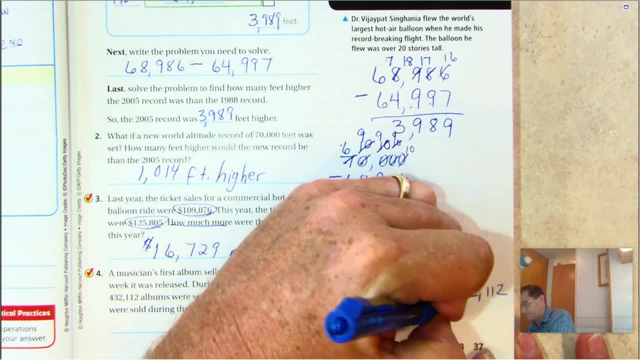 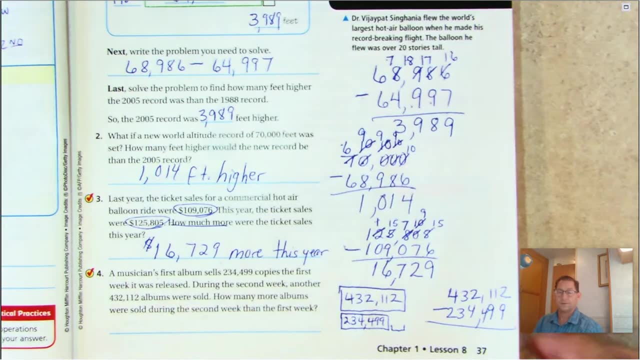 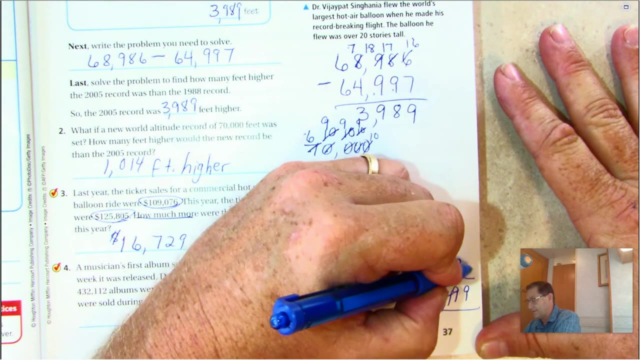 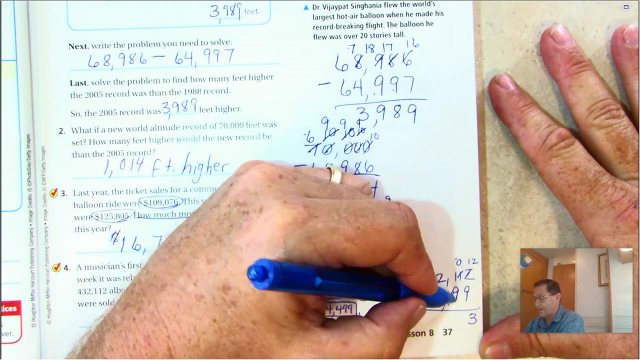 So we are subtracting. Line up your place value. Okay, I can't take nine from two ones, So I'll regroup the one ten as no tens Ten ones. Well, take away nine is three ones. Zero. take away nine tens. 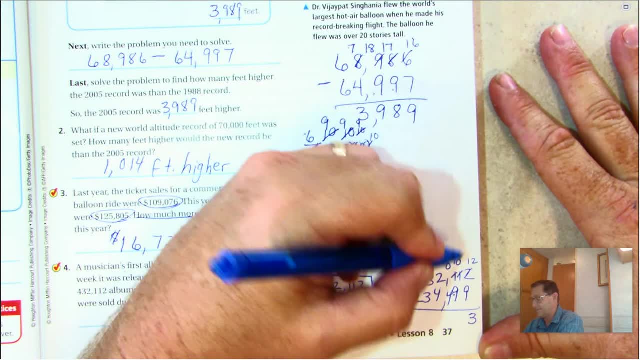 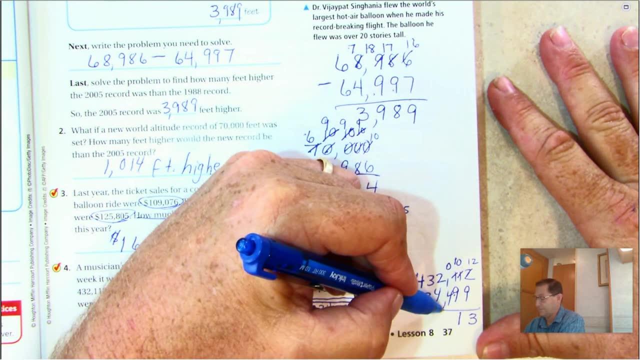 I can't do that. I'll rename the one hundred as no hundreds and tens Ten. take away nine. tens is one ten Zero. take away four hundreds. Can't do that, So I'll rename the two thousands as one thousand and ten hundreds. 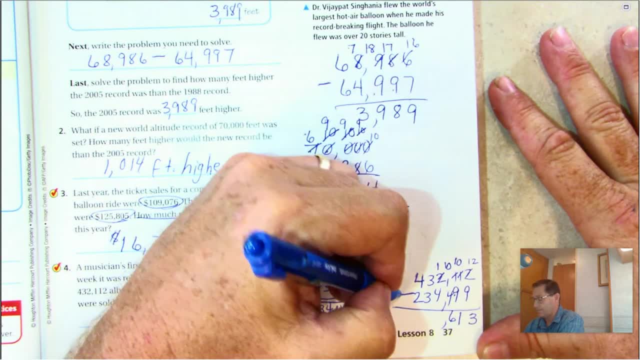 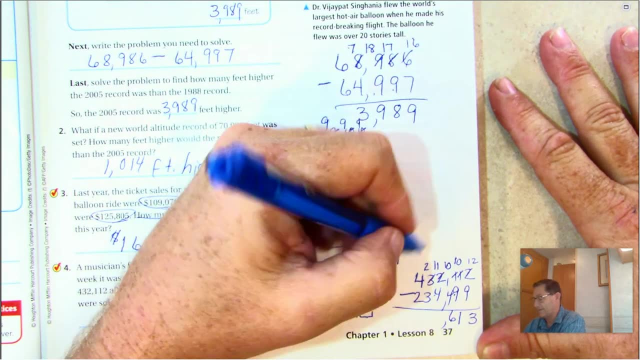 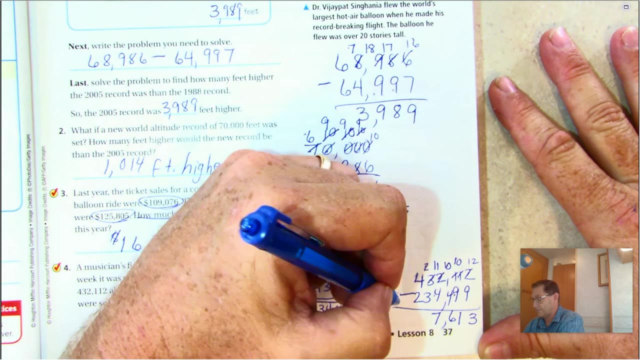 Ten take away four. hundred is six hundred. One thousand, take away four thousand. I can't do So. I'll rename the three, ten thousands as two, ten thousands and ten hundreds. So eleven take away four is seven thousand. Two, ten thousands, take away three cannot do. 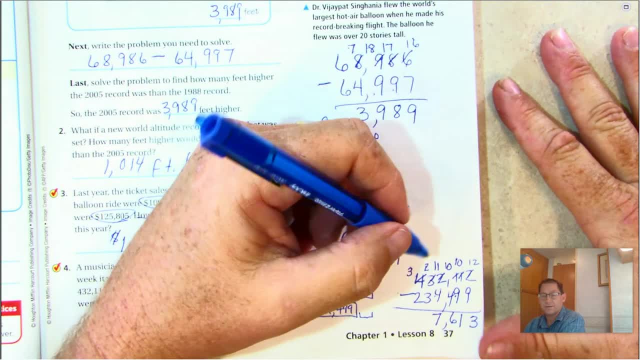 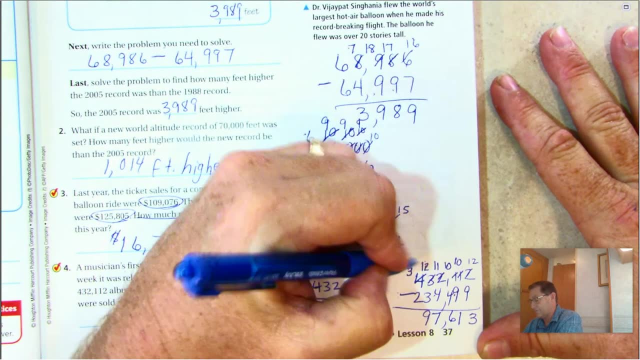 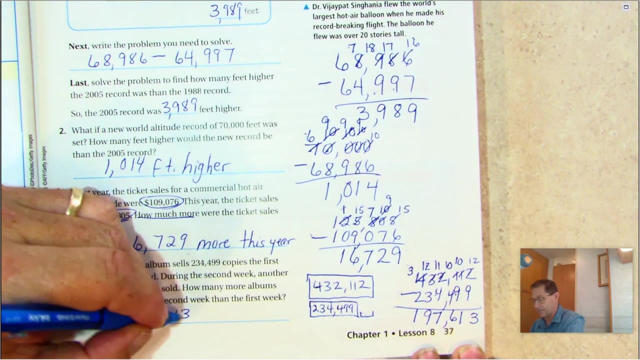 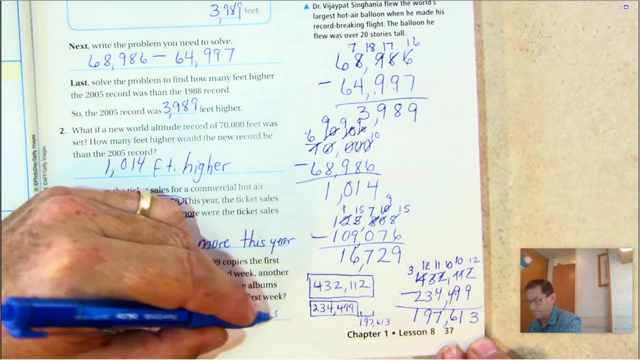 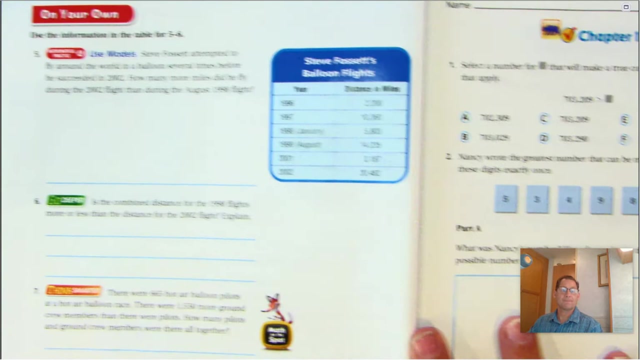 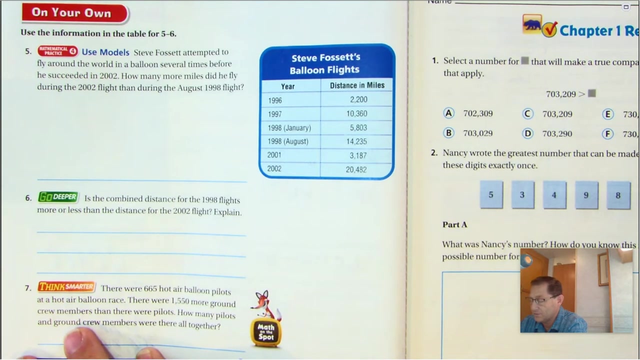 So I'll rename the four hundred thousand as three hundred thousand and ten ten thousands Twelve. take away three is nine. Three take away two hundred thousand is one, So they sold 197,613 more albums. Number five: Steve Fawcett attempted to fly around the world in a balloon several times before he succeeded in 2002.. 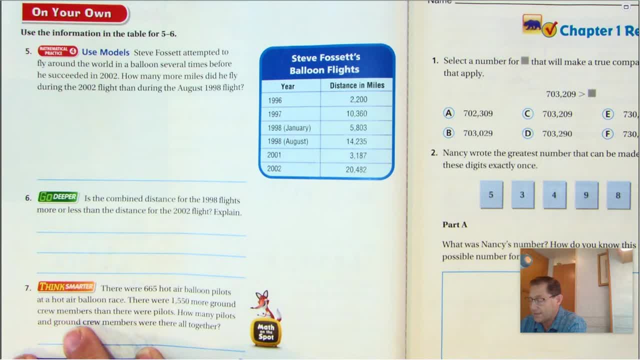 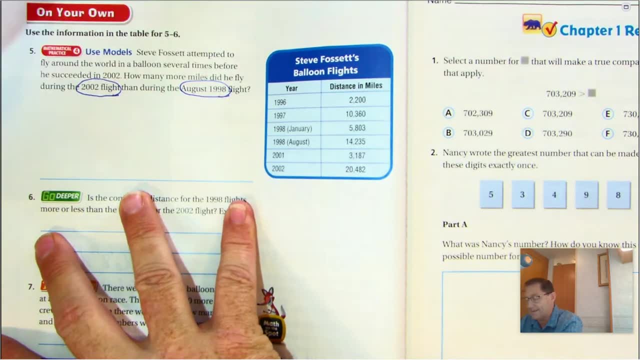 How many more miles did he fly during the 2002 flight than the August 1998 flight? So I need 2002 and 1998.. And our information up here says: use the table for numbers five and six. So these are his balloon flights. 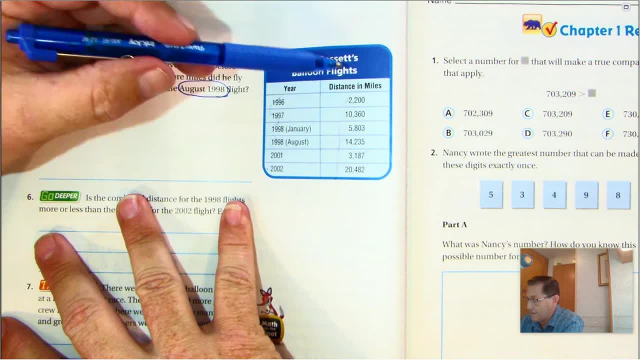 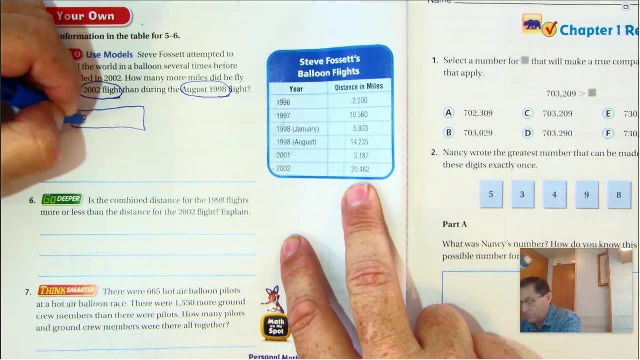 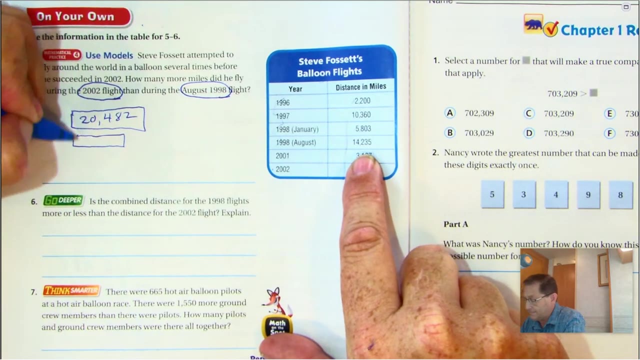 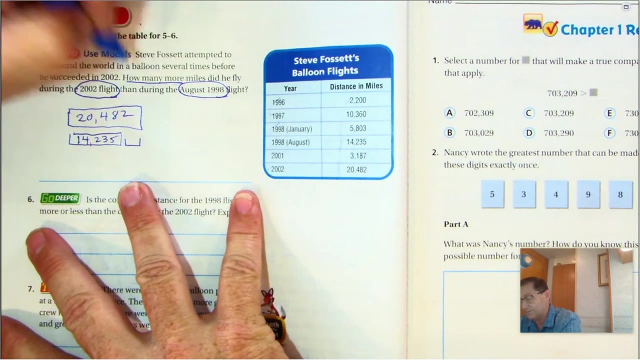 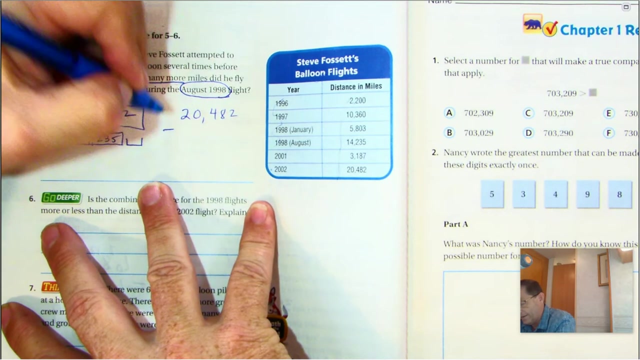 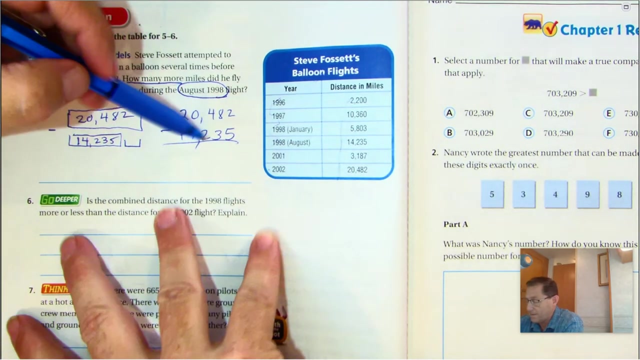 These are the years and these are his distances in miles. So his 2002 flight was 20,482.. His August 1998 was less And it wants to know how many more miles. So that would be subtract 20,482, take away 14,235. 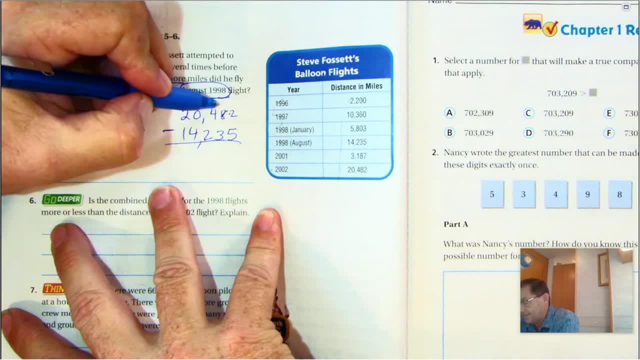 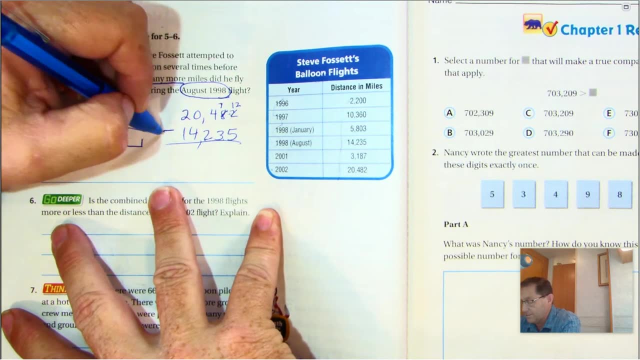 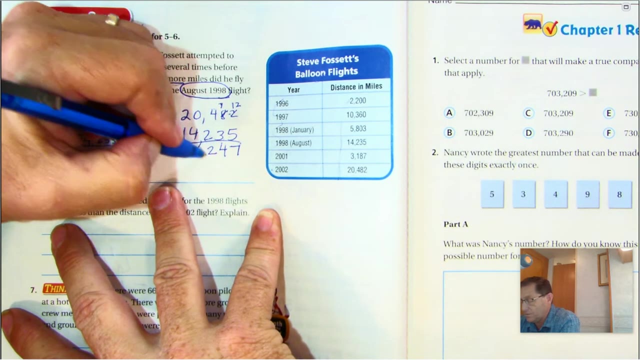 We can't take five from two ones, So I'll rename the eight tens as seven tens, One ten And ten ones. Twelve ones: take away five is seven ones. Seven tens. take away three tens is four tens. Four hundred. take away two hundred is two hundred. 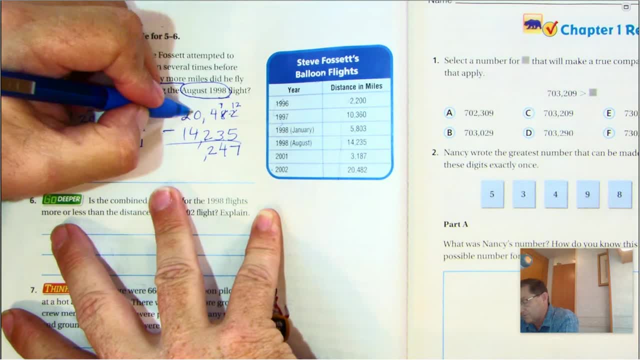 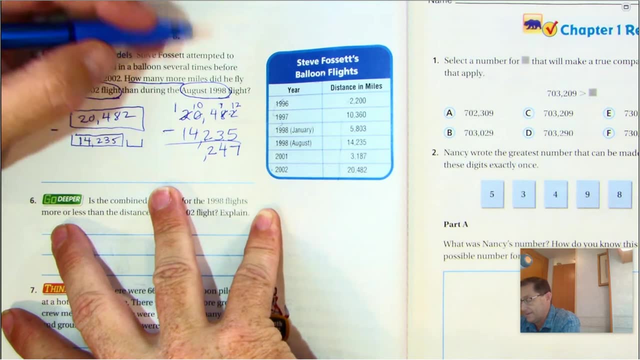 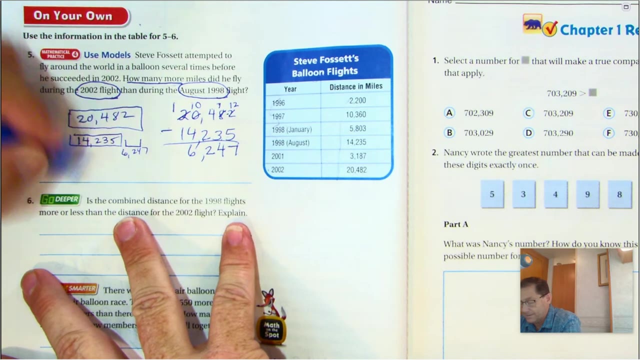 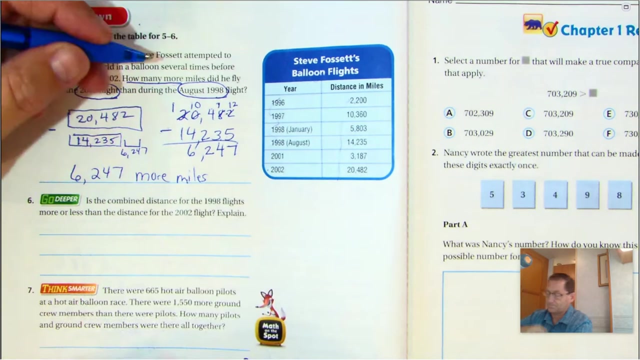 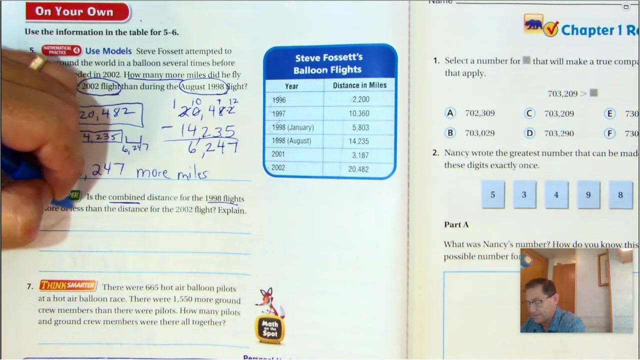 I can't take four thousand from zero thousands, So I'll rename the two thousand, ten thousands as one, ten thousand and ten thousand ones. Ten. take away four is six, So Six thousand two hundred forty seven thousand more miles. Number six Is the combined distance for the 1998 flights, more or less than the distance for the 2002 flight. 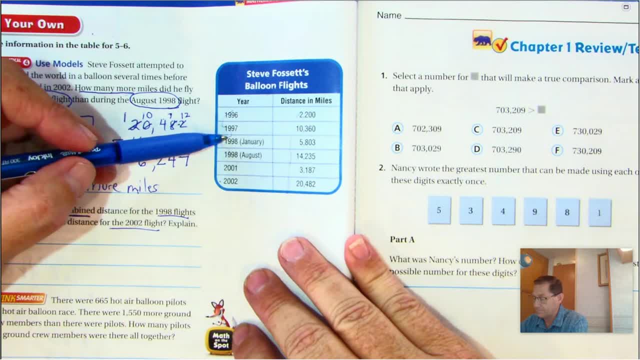 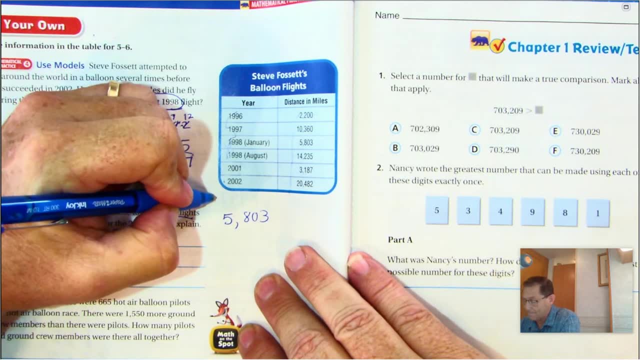 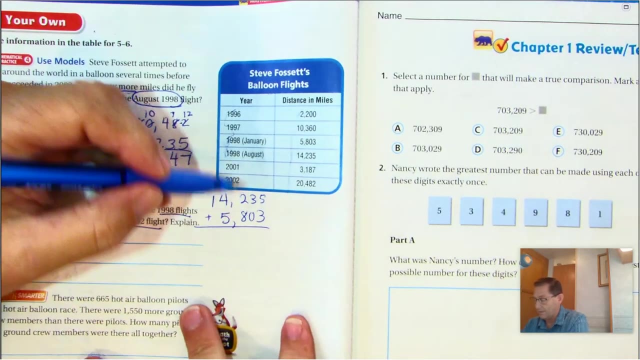 So the 1998 flights. When I look at the table I see that there's two dates. So combined means to add Okay. So I need to make sure my place values lined up And they are. I'm going to add five and three is eight. 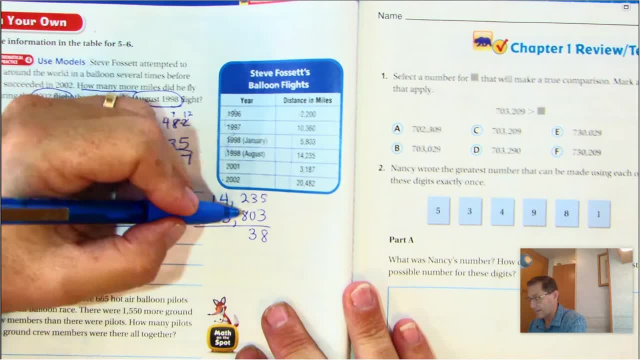 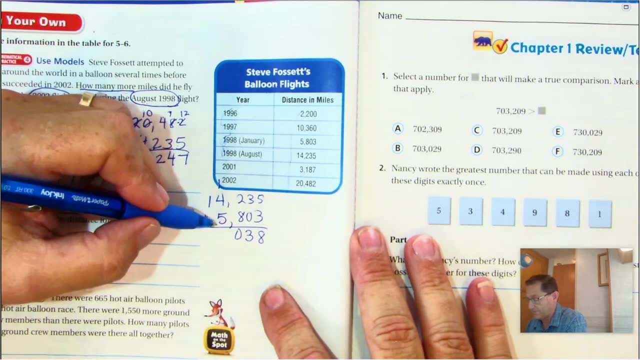 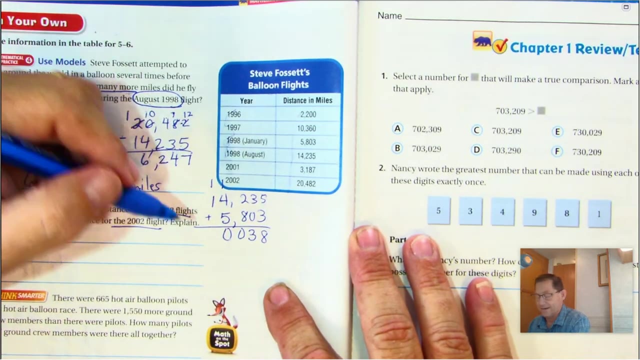 Three tens and no tens is three tens. Eight hundred and two hundred is ten hundred, which can be renamed as one thousand, And zero hundred Five plus four is nine, Plus the regroup thousand is ten thousand, Which can be renamed as one hundred thousand. 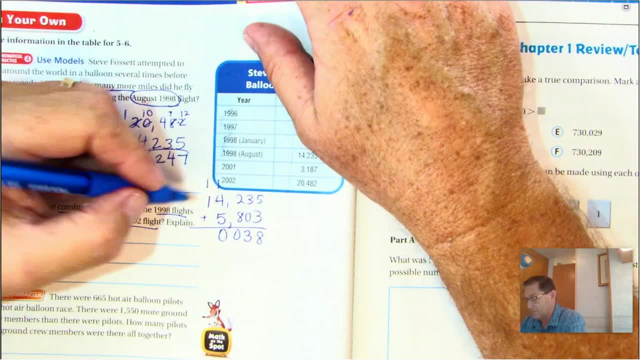 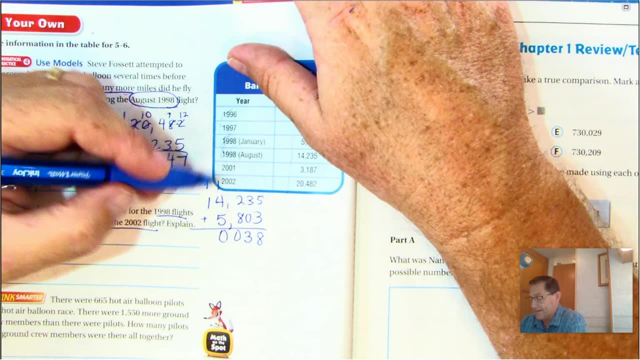 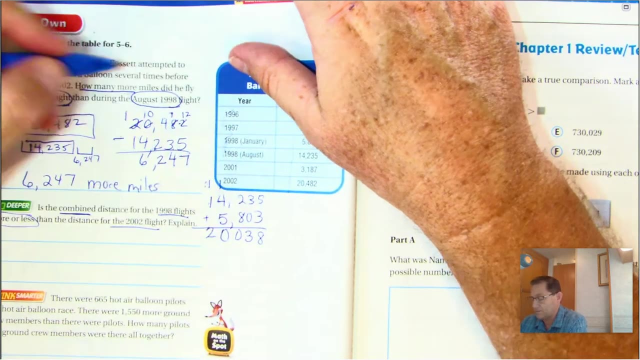 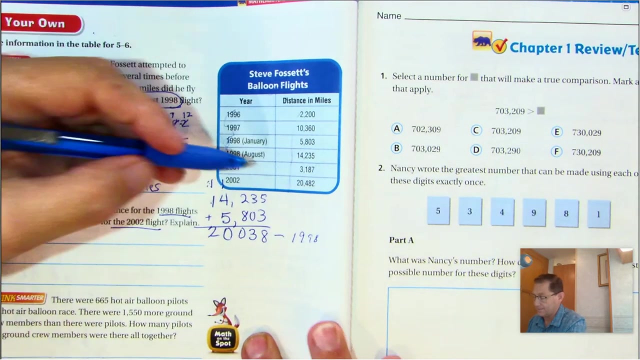 And zero ten thousand. One hundred thousand plus one. Sorry, Ten thousand can be renamed as one ten thousand And zero thousands. One ten thousand plus one ten thousand is twenty thousand. So Combined. These are the 1998 flights. The 2008 flight is twenty thousand four hundred eighty two. 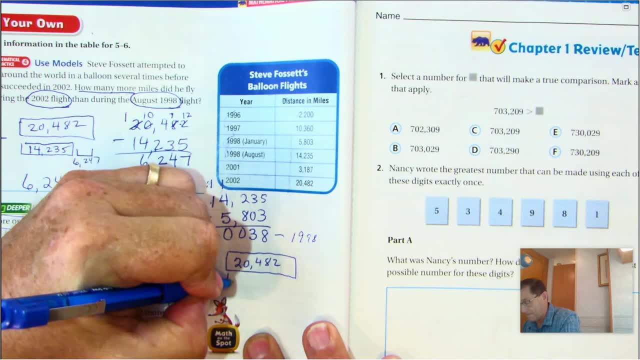 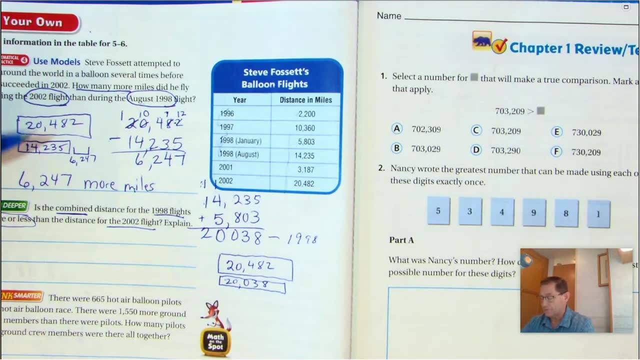 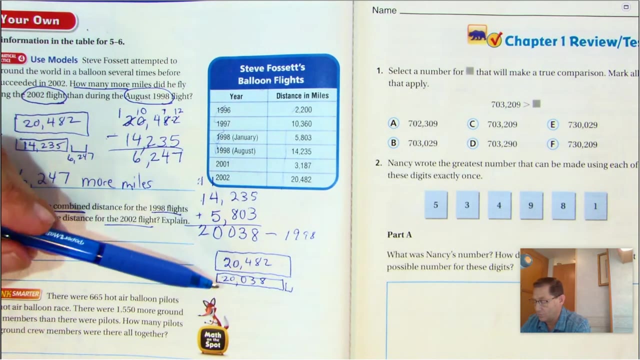 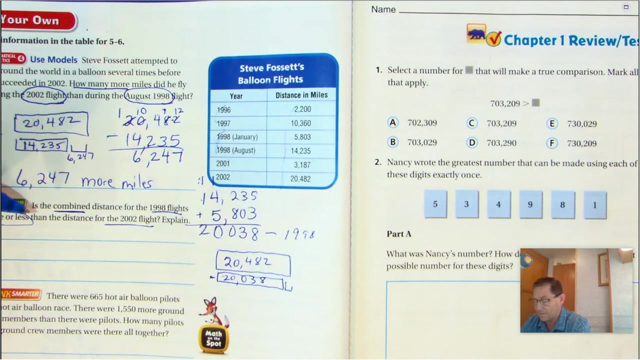 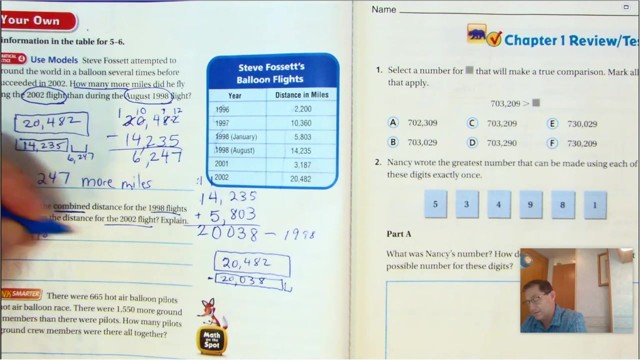 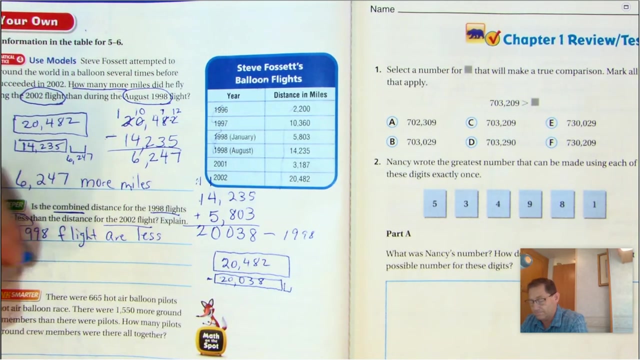 Eighty two, So Two thousand two. Twenty thousand four hundred eighty two Is greater than twenty thousand thirty eight. So is the combined distance for the 1998 flights More or less So the 1998.. Flights are less than the two thousand five hundred ninety-six. 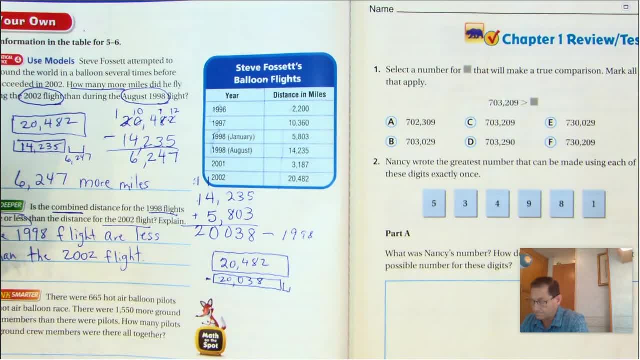 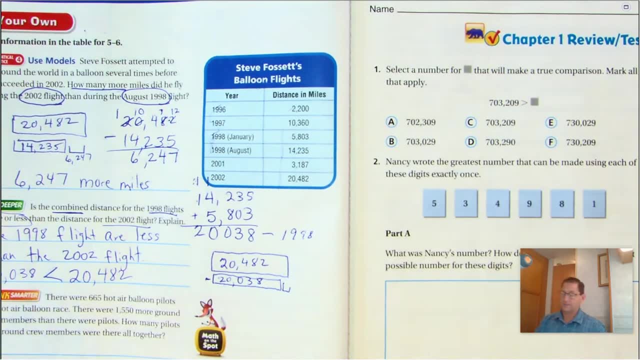 So the 1998.. Flights are less than the two thousand seven hundred. It's thirty thousand, Twenty thousand two hundred and thirty eight From the early 1990.. And this is the annual gain, This is the annual gain, The annual gain. 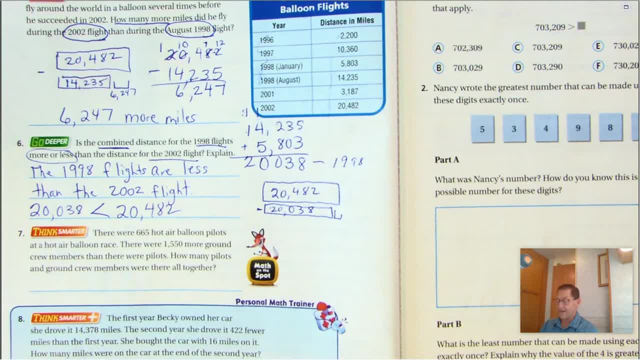 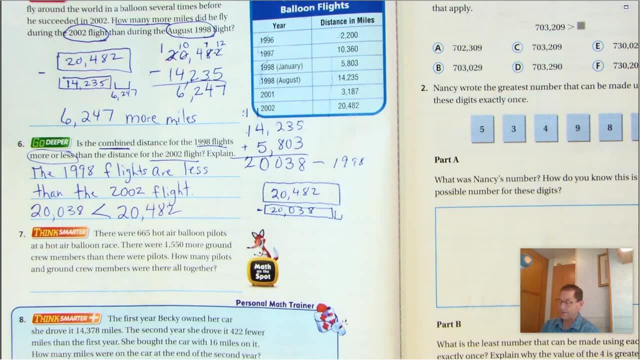 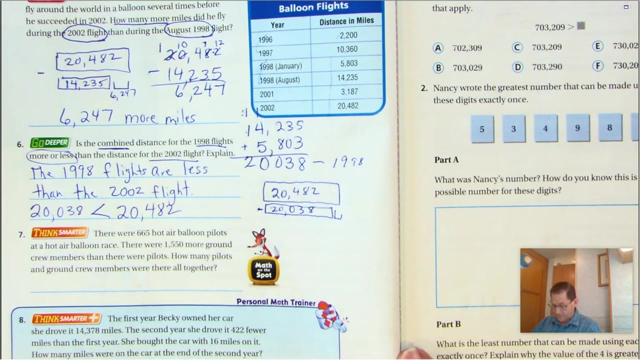 less than the 2002 flight, because 20,038 is less than 20,482.. Number seven: there were 665 hot air balloon pilots. at a hot air balloon race, There were 1,550 more ground crew members than there were pilots. How many pilots and ground crew members were there all together? So I noticed. 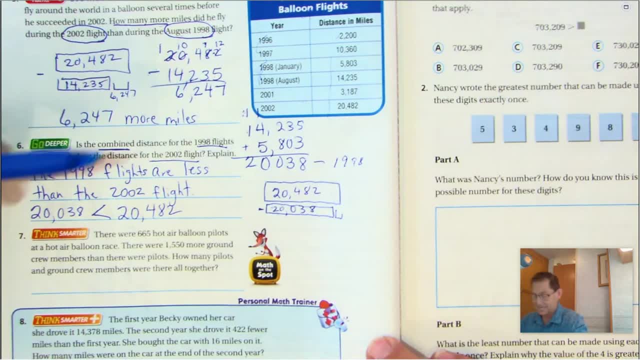 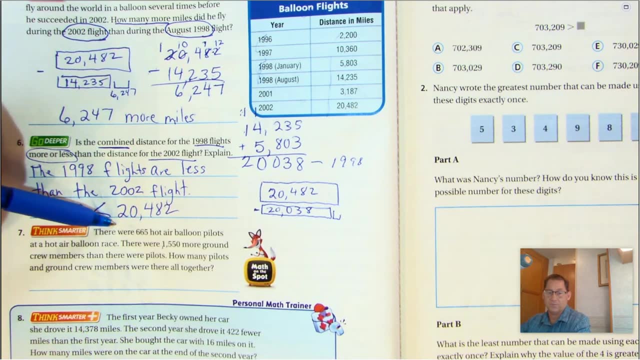 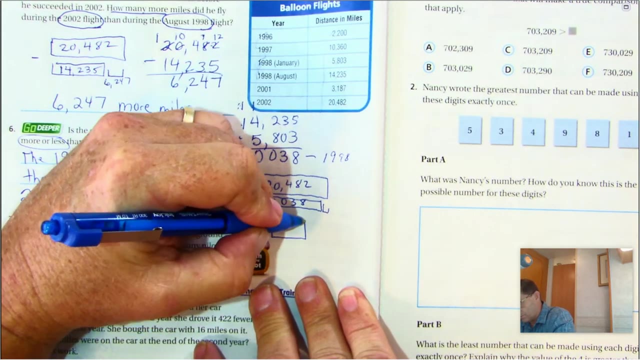 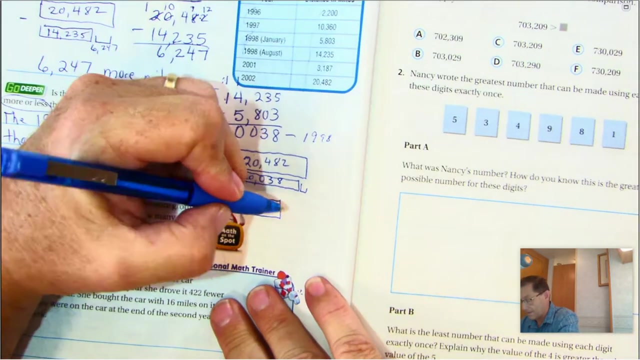 this is going to be a two-step problem, because they didn't actually give me the total amount of ground crew members. They just told me that it was this many more than the hot air balloon. So we have 665 hot air balloon pilots plus 15,000. 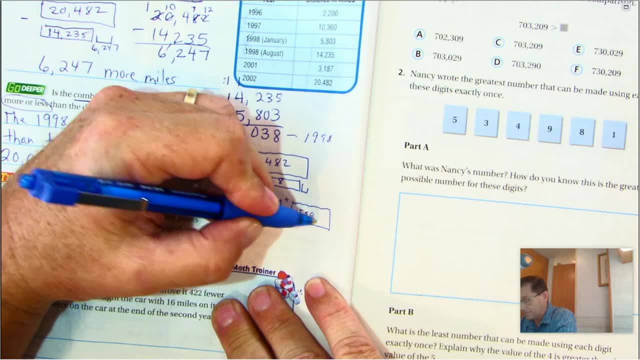 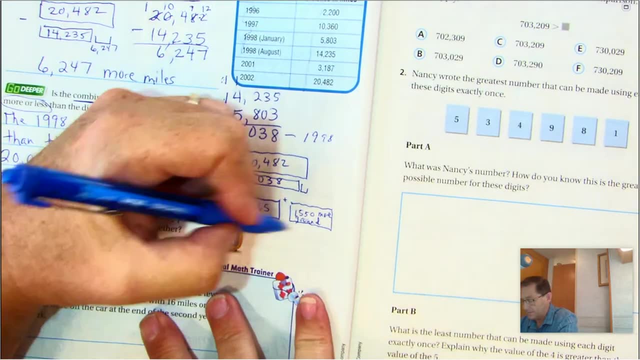 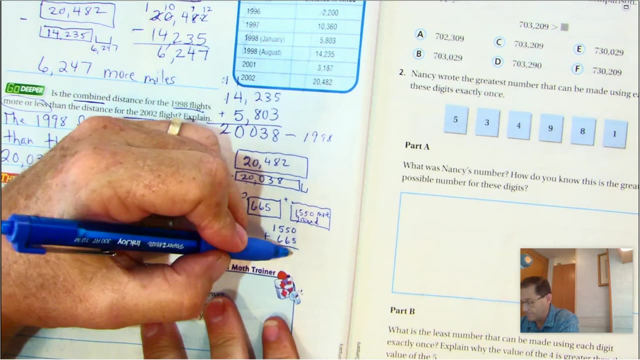 ground, more ground. So to figure out the number of ground members I'm going to have to add So 1,550 plus 665.. My place values lined up So five, six tens and five tens is 11,, 10.. Rename that as. 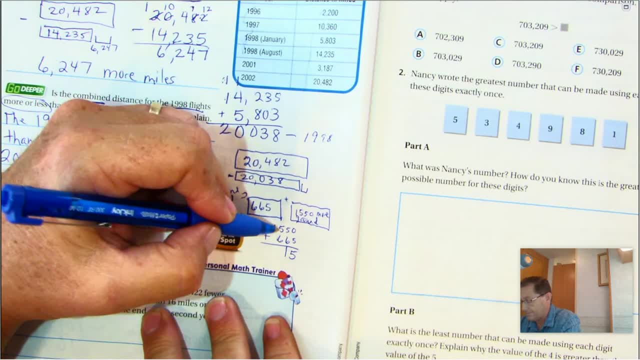 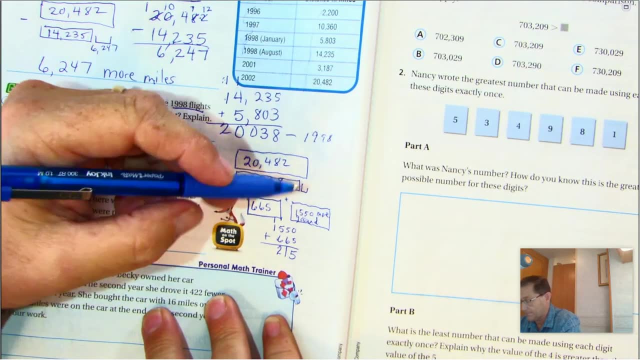 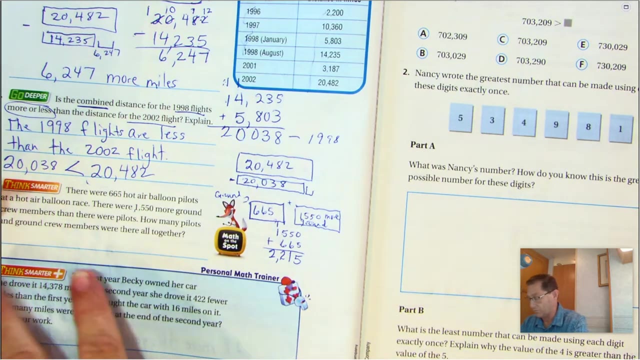 100 and 110.. Six and five is 11. again plus one more is 12.. So 1,200 can be renamed. There's 1,125 ground crew members and a 16,000 ground crew members combined as and includes 21,200 ground crew members. But封Mukoo's map said the max number of ground crew members show. 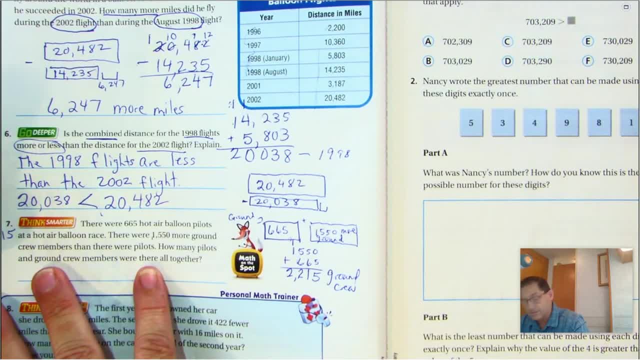 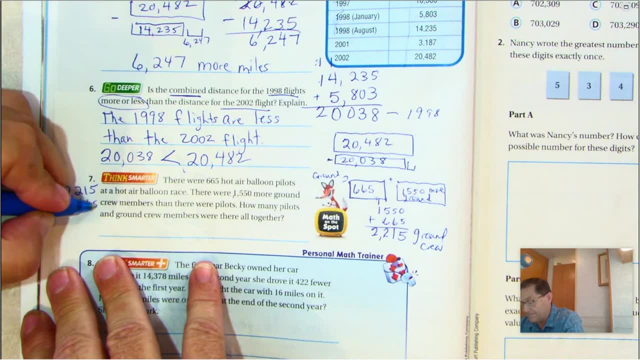 well, when the number of ground crew members is equal to two and then the total number of ground crew missions is covers, So 2,215 ground crew members are together, then this total will have each one correct. So unit quarter is ruled as two. So there's 2215 ground crew members. so now we can combine the 2,215 ground crew members and the 665 hot air balloon to find out how much there were all nochmal. 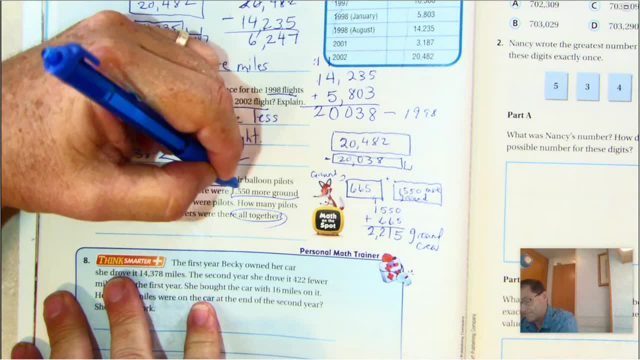 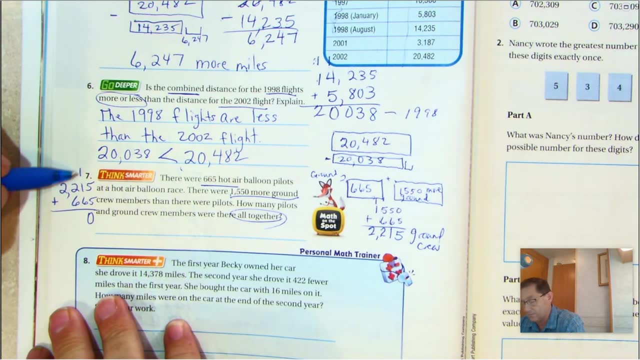 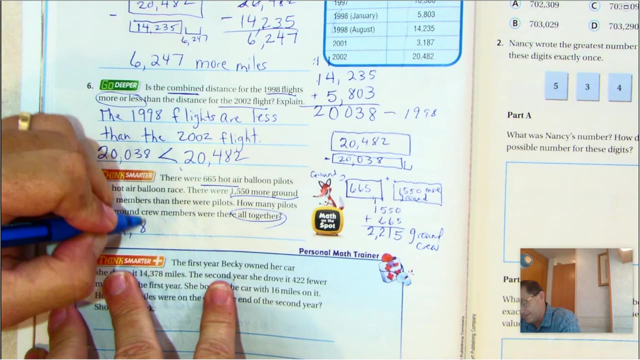 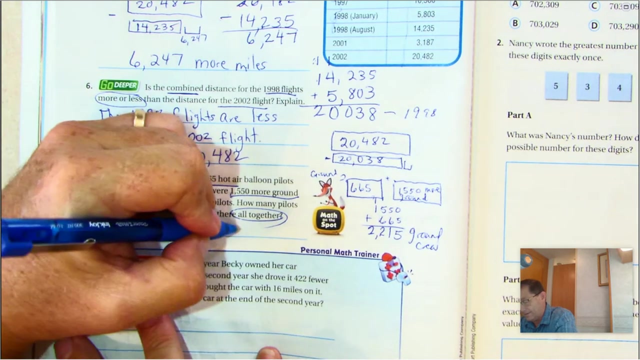 5 and 5 is 10.. Regroup and rename that as 110, 0, 1.. 610 plus 110 plus 110 is 8 tens. 600 plus 200 is 800 plus 2,000.. 2,880 pilots and ground crew. 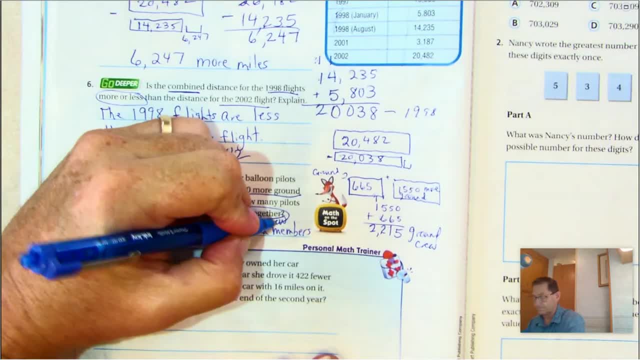 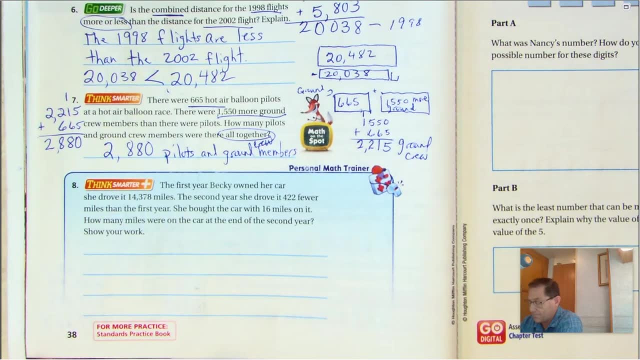 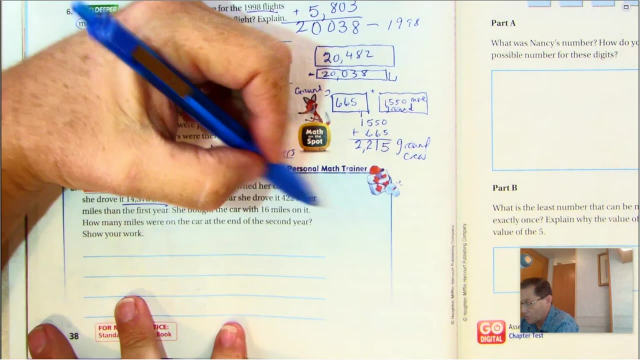 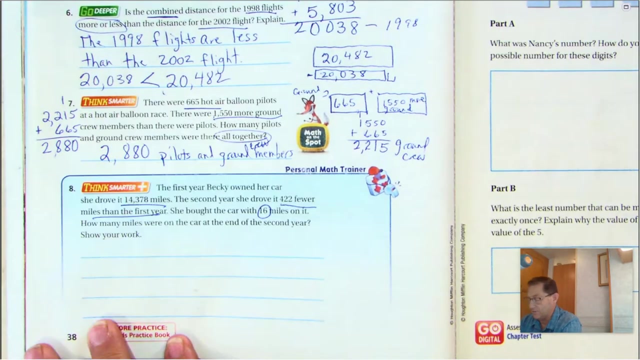 Ground crew members: All right number eight. The first year Becky owned her car she drove it 14,378 miles. The second year she drove it 422, fewer miles than the first year. She bought the car with 16 miles on it. 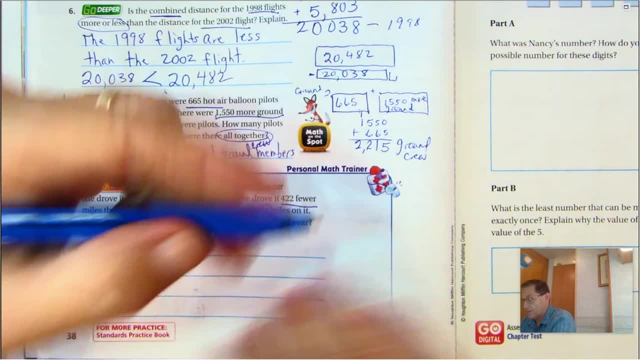 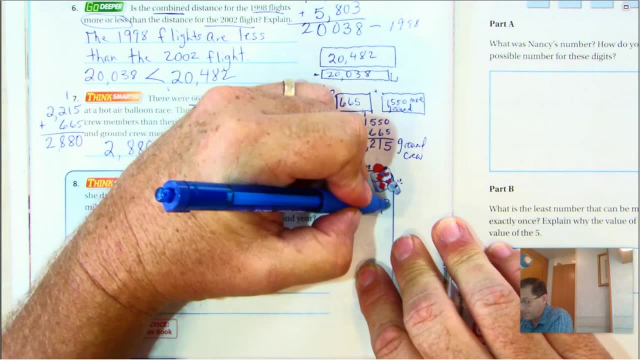 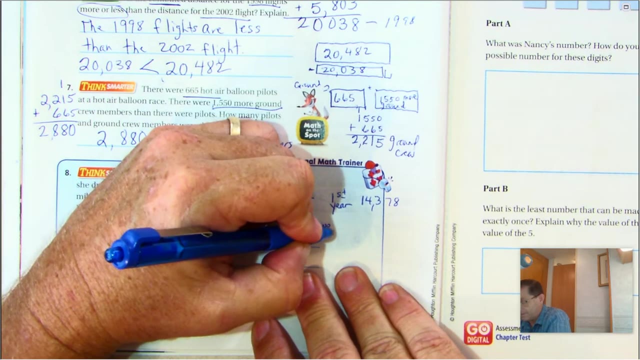 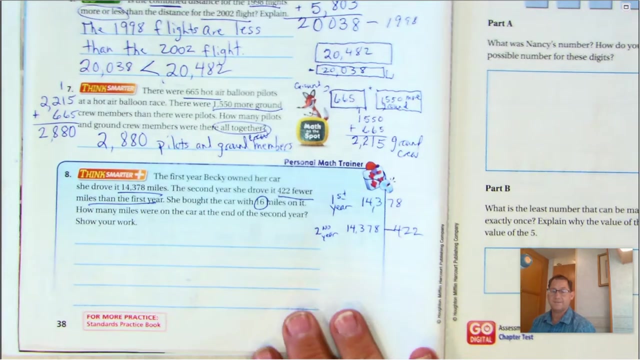 How many miles were on the car at the end of the second year. So we're given that the first year was 14,378.. We have to figure out the second year. So the second year was 422 fewer than the first year. 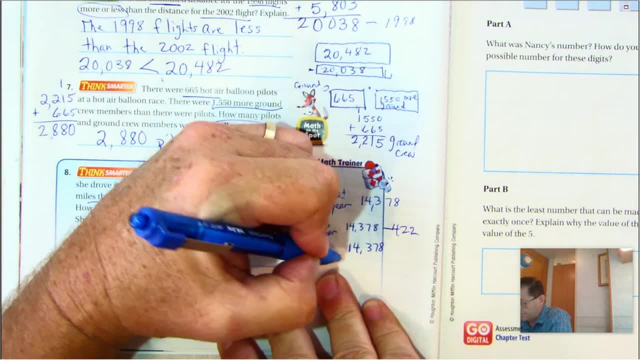 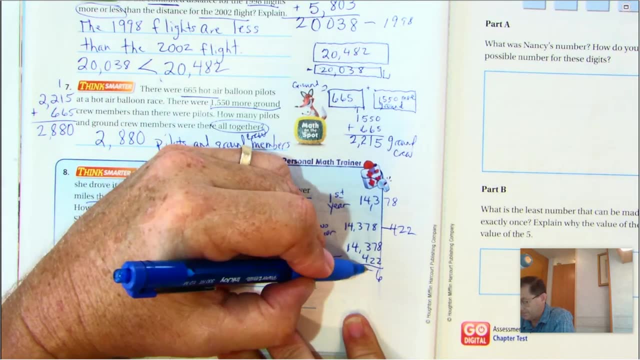 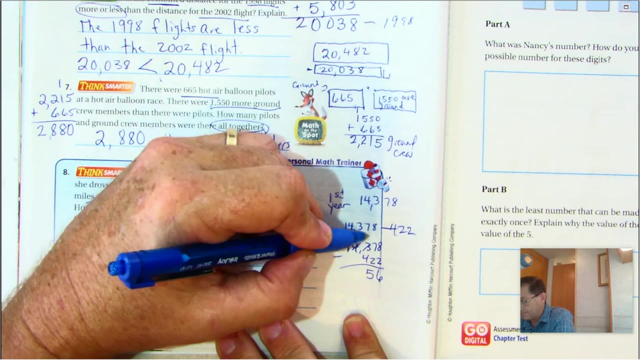 So let's subtract those Eight takeaways. Two is 6, 1.. Seven tens take away two. tens is 5.. I can't take 400 from 300, so I'm going to rename that as 3,000 and 10 hundreds. 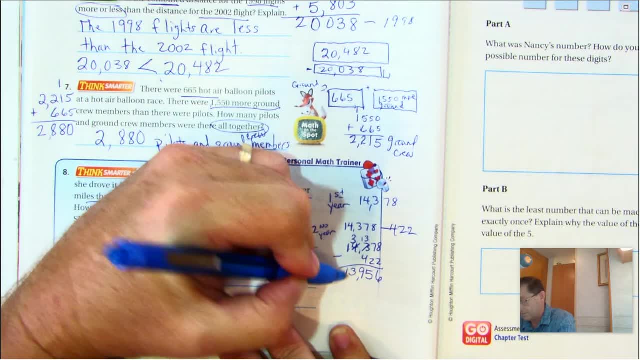 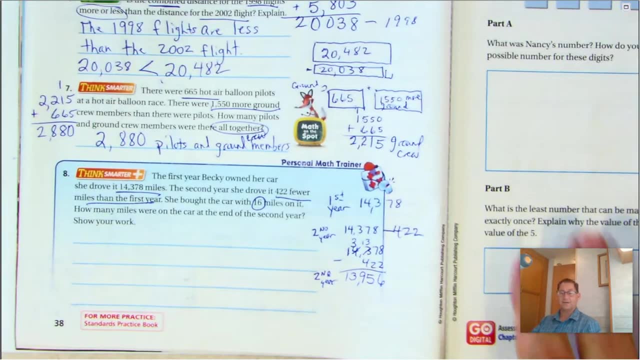 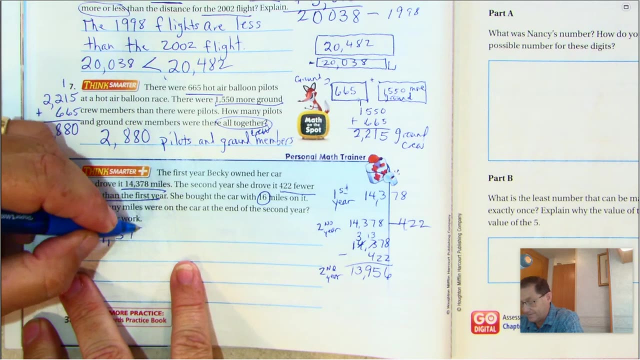 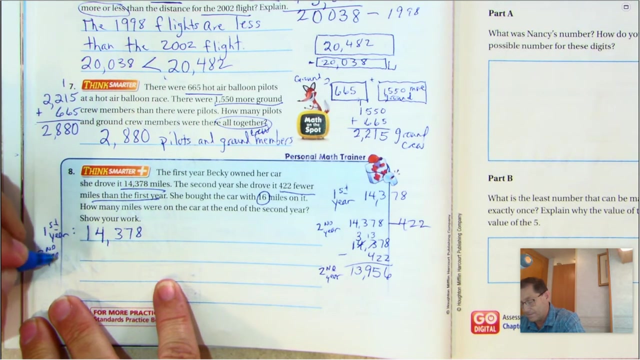 13. take away 400 is 900.. Okay, so the second year she drove 13,956.. So now we're going to combine all Three numbers that we need, So first year plus the second year plus the 16.. 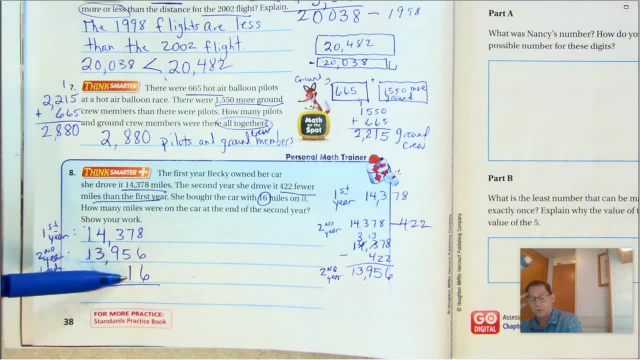 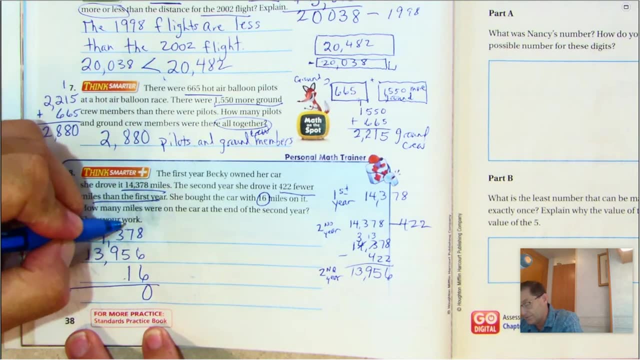 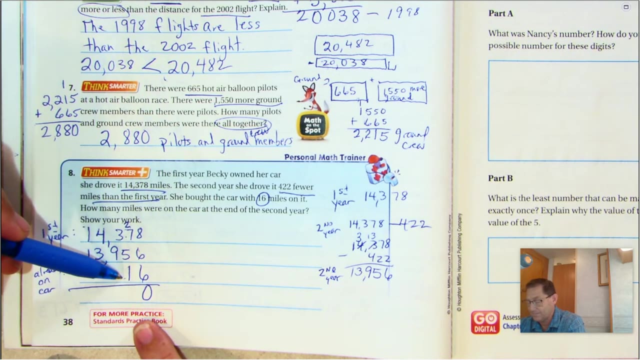 Okay, So first year, second year plus the 16.. Now we're already on the car right: Six and six is 12, plus eight more is 21.. I'll rename that as two tens and no ones. Seven and two more is nine plus one is 10, plus five is 15.. 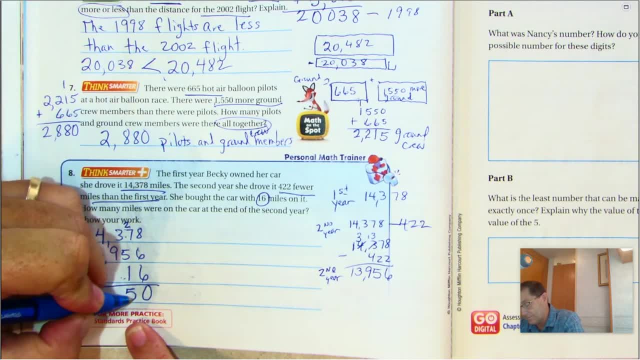 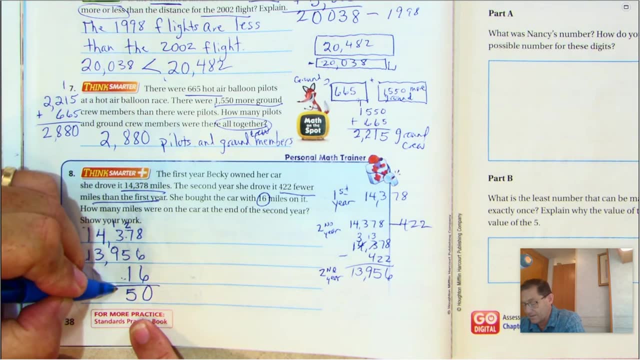 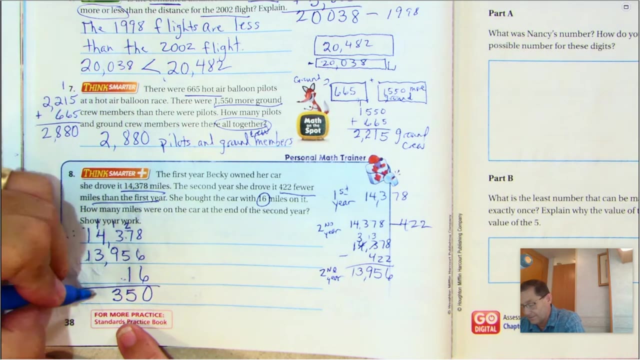 So 15 tens will be renamed as 100, and five tens- 900 plus 100- is 10, plus three more is 1,300.. I'll rename that as 1,300.. 4,000 plus 3,000 plus 1,000 is 8,000.. 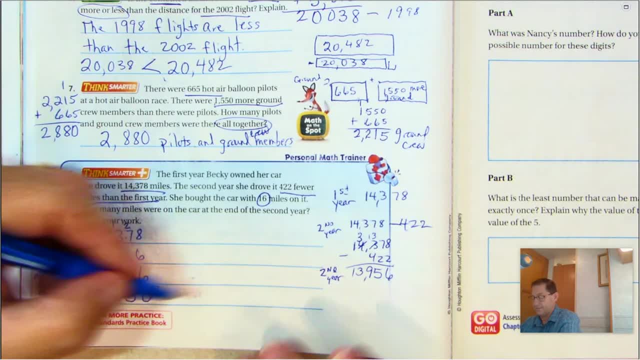 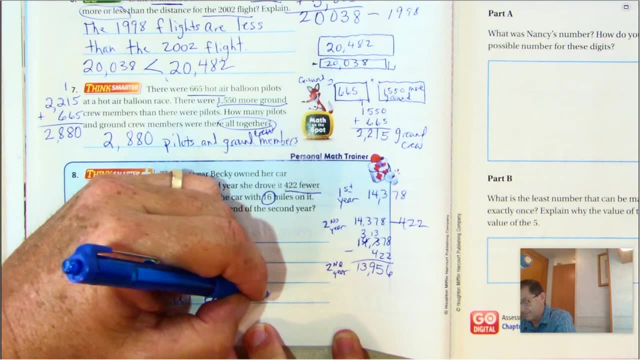 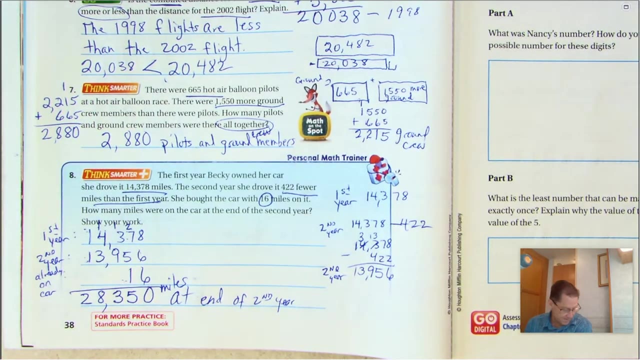 10,000 plus 1,000, 10,000, 28,000.. So Becky has 28,350 miles at the end of her second year. Okay, so that's it for our lesson on 1.8.. 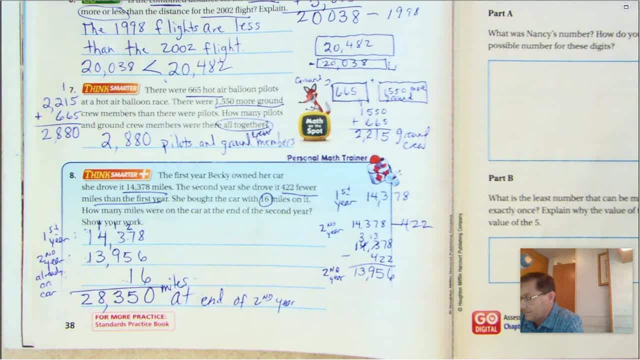 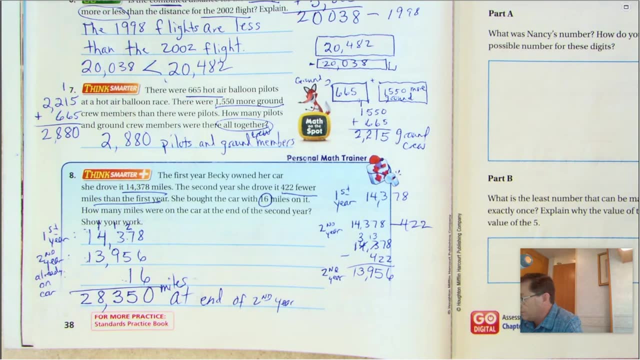 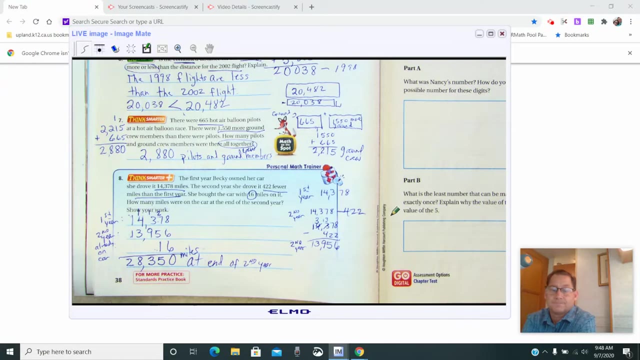 We have completed Chapter 1.. So the next thing we'll be doing is the Chapter 1 review to practice for our test, And so until we do the Chapter 1 review, may the numbers always be in your favor, Thank you.